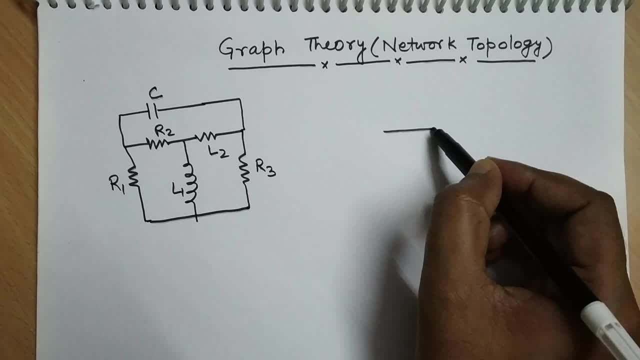 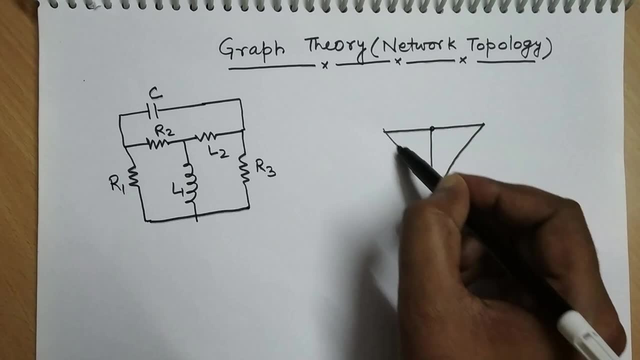 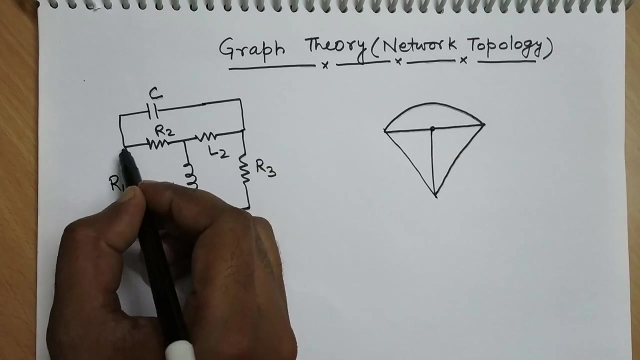 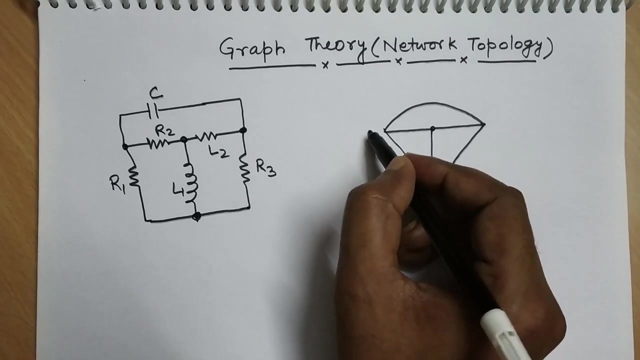 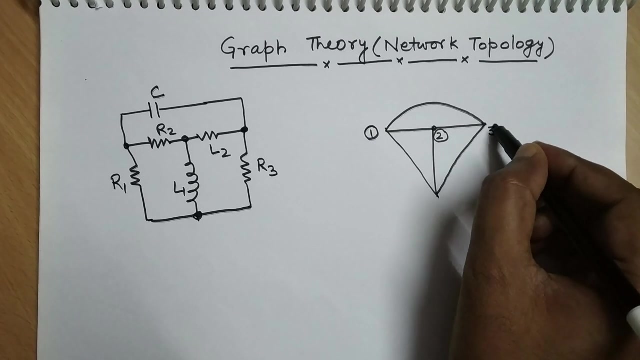 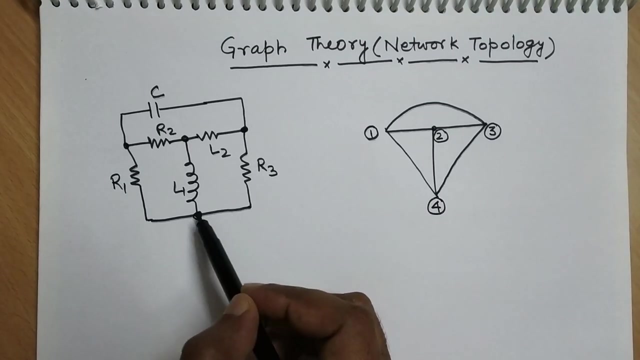 represented as this, by assuming all the interconnecting point as a node. So this is node one, this is node two, this is node three and this is node four. We can observe here that R1, L1 and R3 all are connected at the same point. 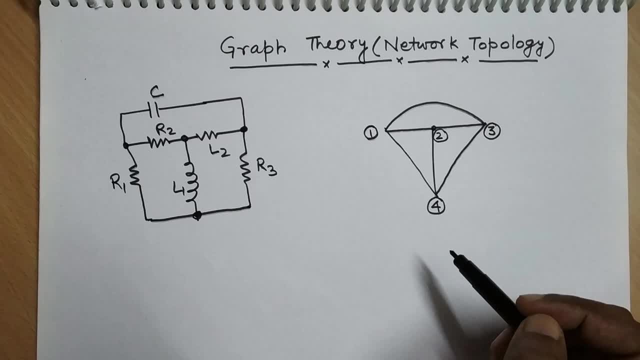 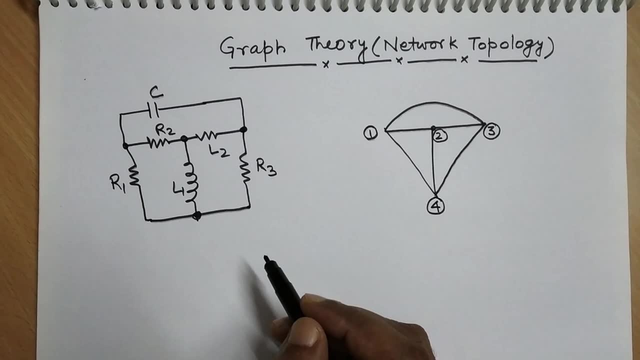 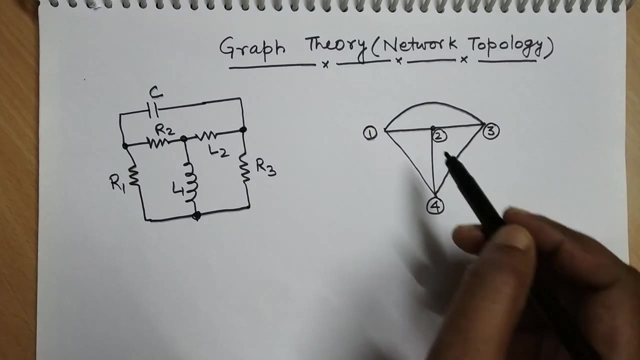 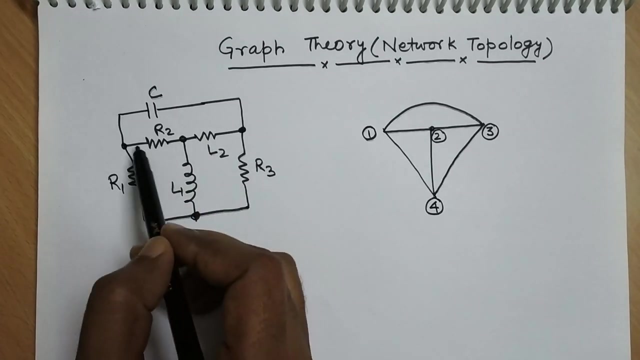 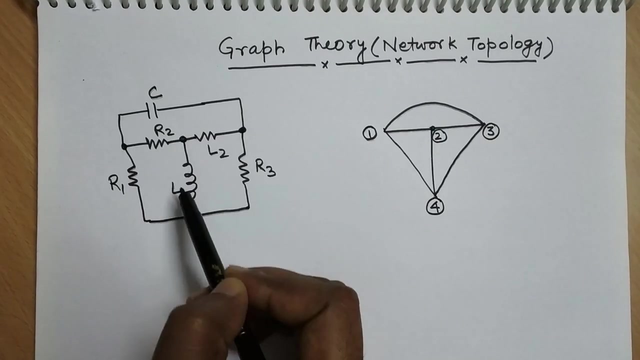 So this is the point four. So there are various terminology in this network graph. The first one is branch. So branch is any elements of the graph is called branch. Let's say R1, so R1 is a branch, R2 or L1, these are called branch And the terminal of these two branches are called nodes. 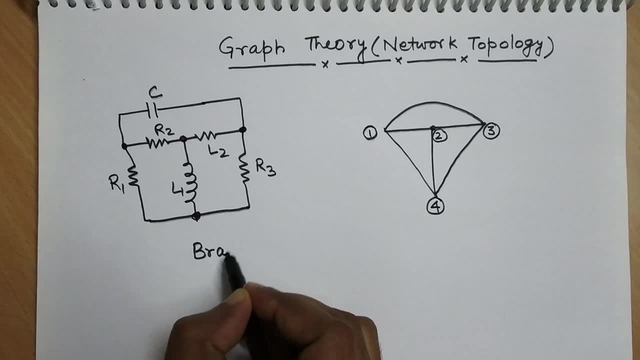 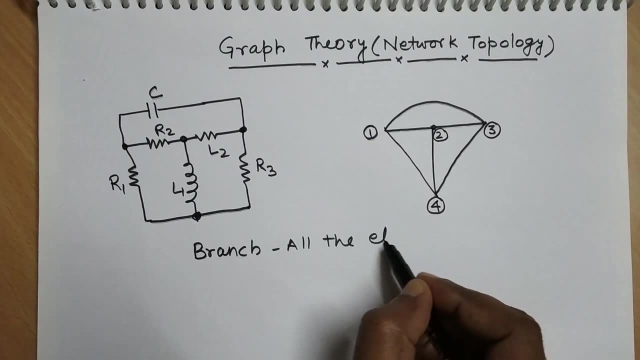 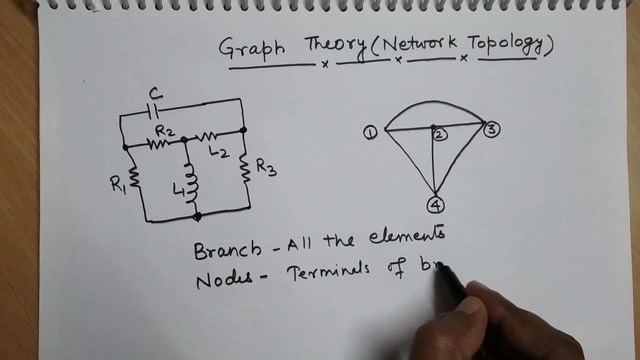 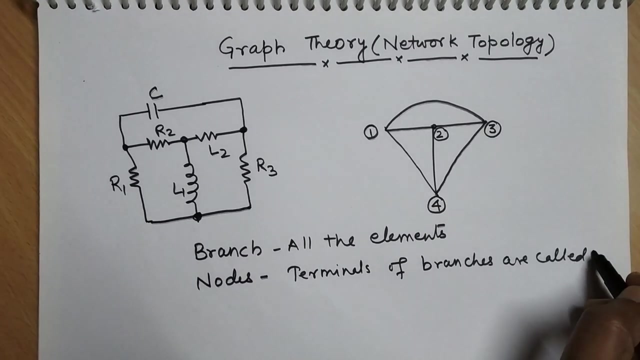 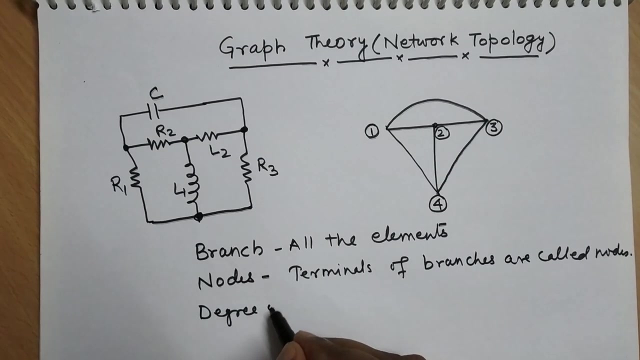 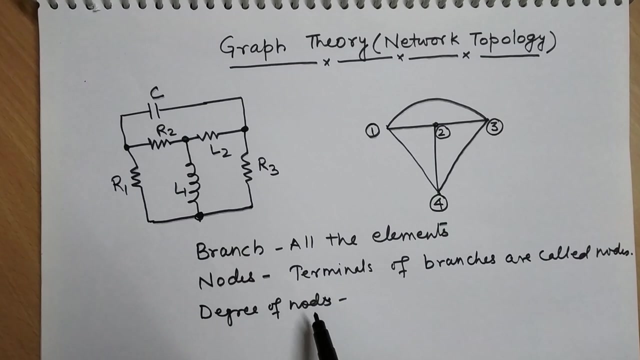 So the first thing will come as branch, So all the elements are called as branch, Then nodes, So the terminals of branches are called nodes. now the third one is degree of nodes. so the degree of nodes is number of branches connected to a network. let us say, at this node, node number four, there are three branches connected, so the 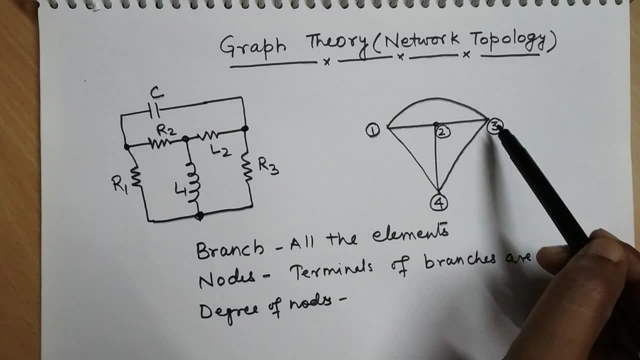 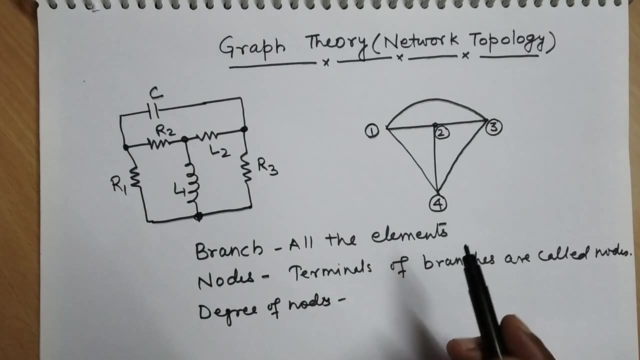 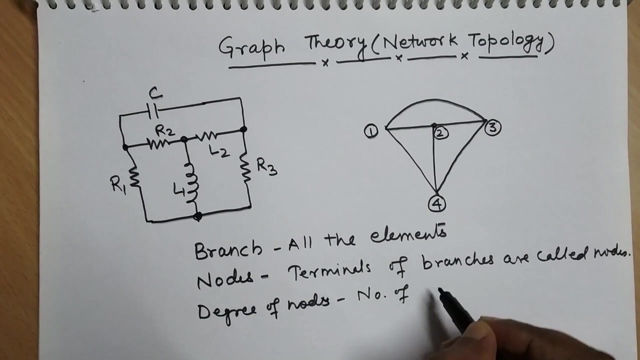 degree of nodes is three. if we take node three, then there are again three branches connected, so degree of these nodes is three. similarly, if you have only two branch connected at a node, the degree of nodes is two. so degree of nodes is number of branches connected to a network. 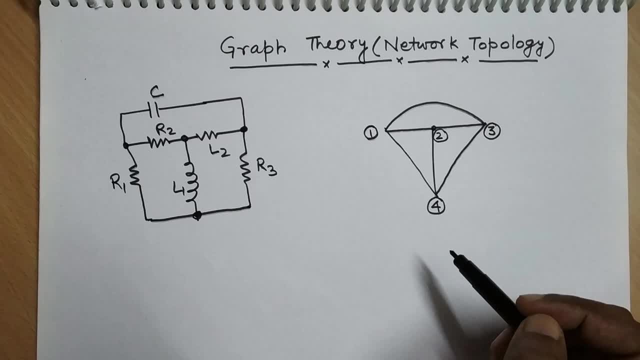 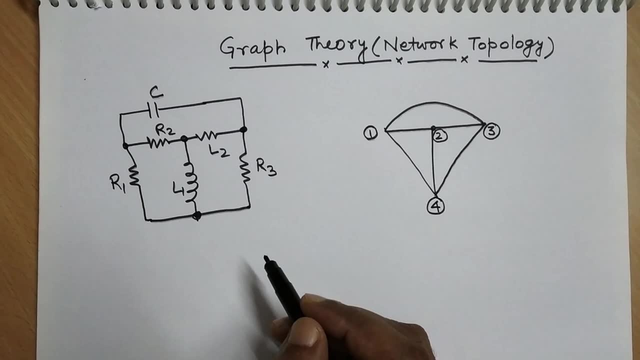 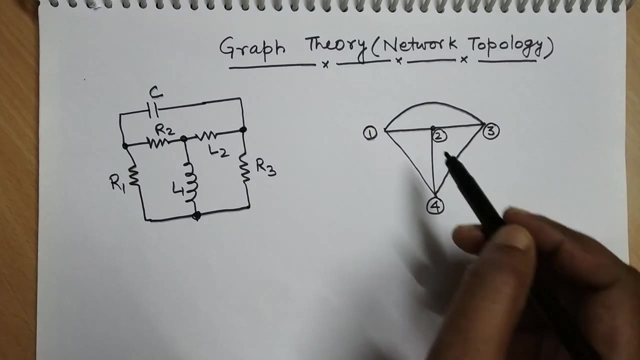 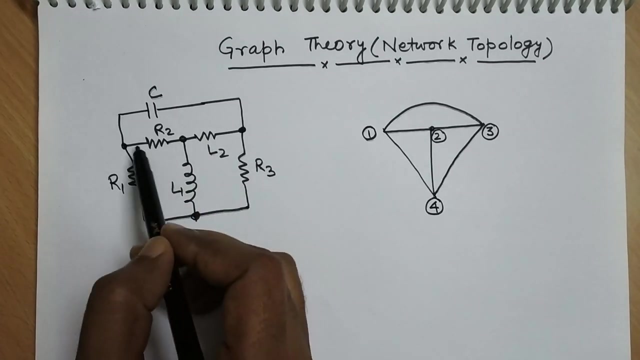 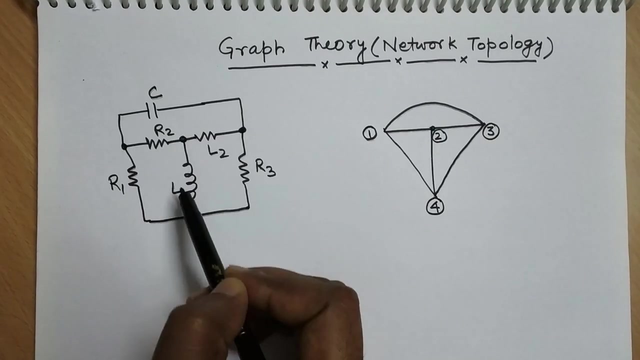 So this is the point four. So there are various terminology in this network graph. The first one is branch. So branch is any elements of the graph is called branch. Let's say R1, so R1 is a branch, R2 or L1, these are called branch And the terminal of these two branches are called nodes. 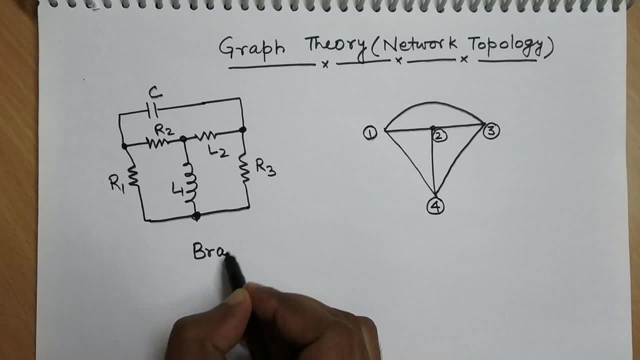 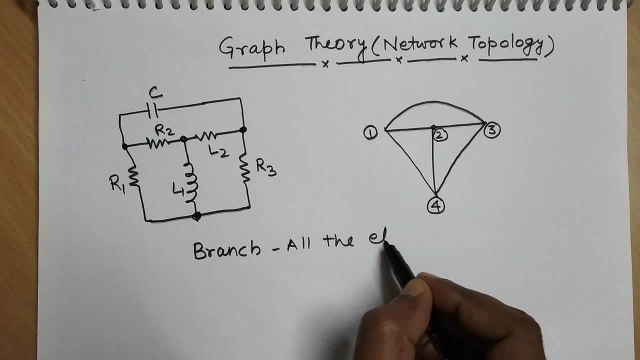 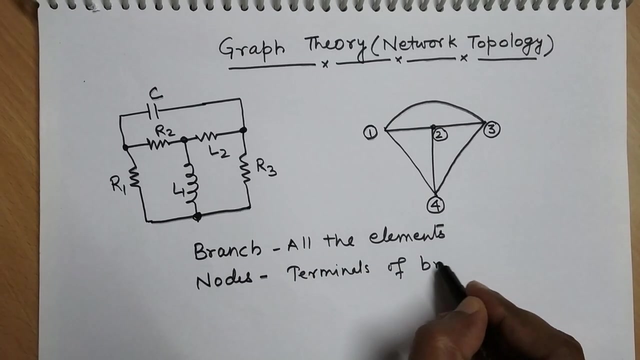 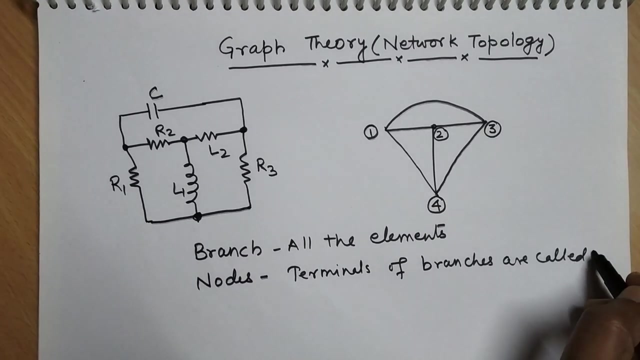 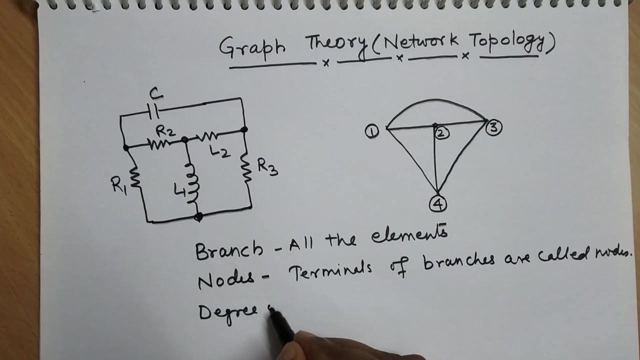 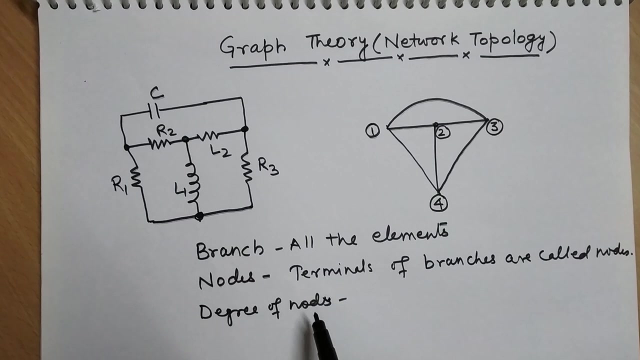 So the first thing will come as branch, So all the elements are called as branch. Then nodes, So the terminals of branches are called nodes. Now the third one is degree of nodes. So the degree of nodes is number of branches connected to a network. Let us say at this node, node number four. 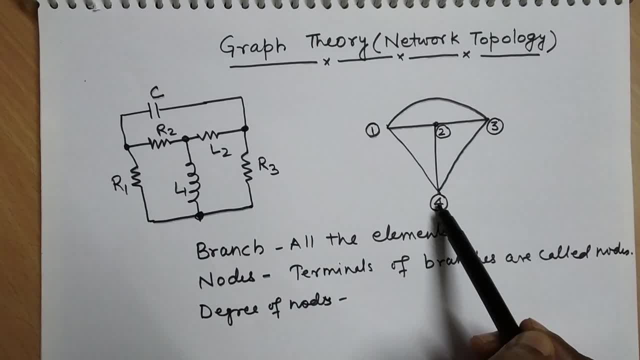 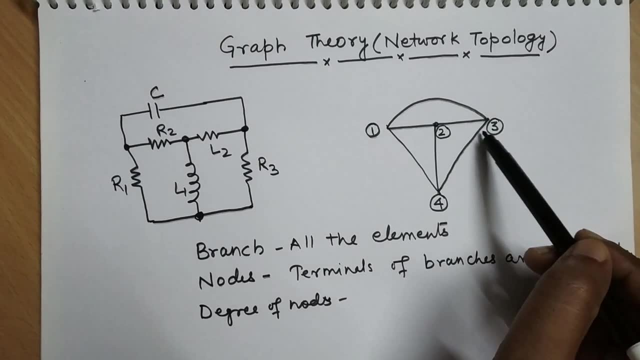 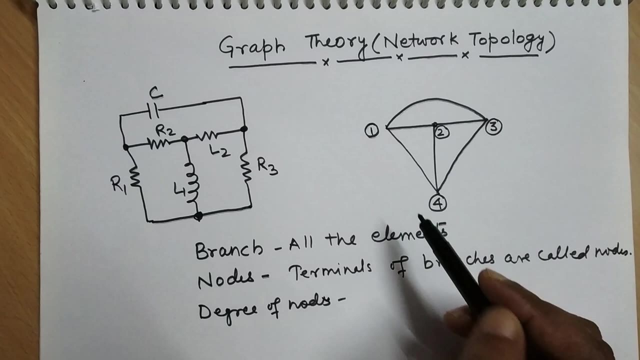 there are three branches connected, So the degree of nodes is three. If we take node three, then there are again three branches connected, So degree of these nodes is three. Similarly, if you have only two branches connected at a node, the degree of nodes is two. 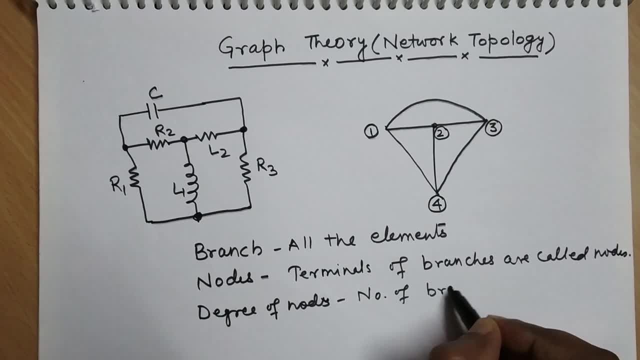 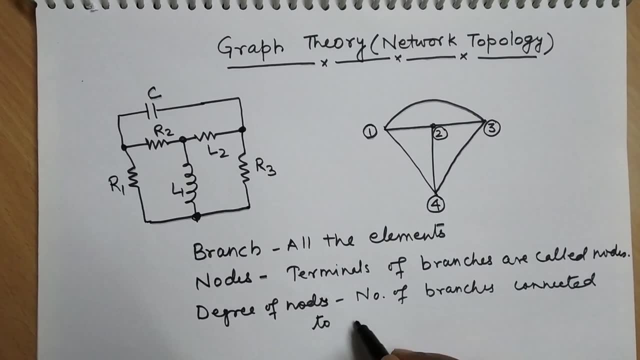 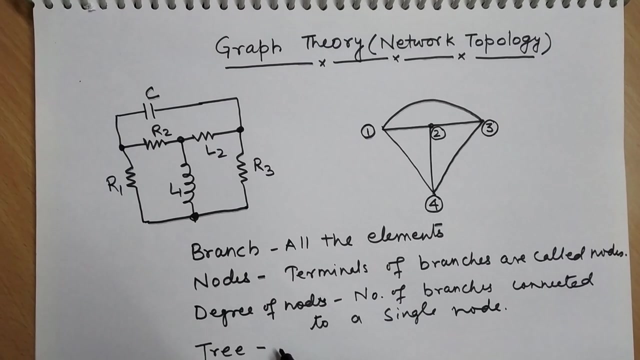 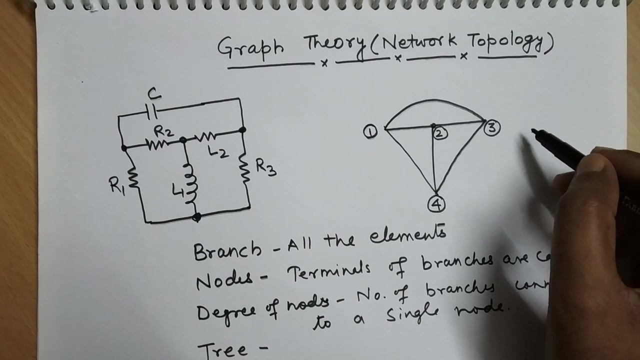 So degree of nodes is number of branches connected to a single node. Then comes the number of branches connected to a single node, This tree, it is interconnected, open set of branches which includes all the nodes of the given graph. So let us take this graph and consider a combination like this. 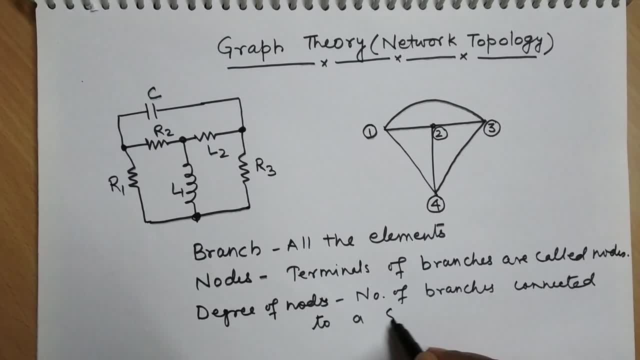 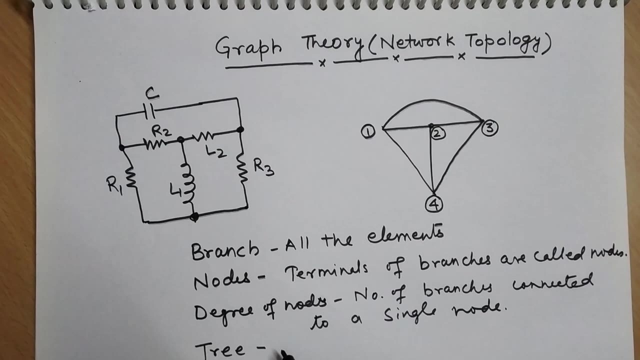 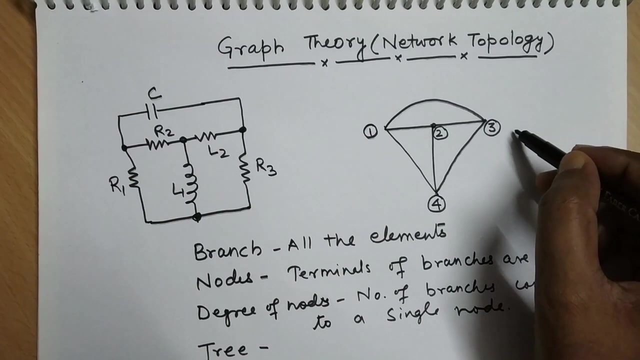 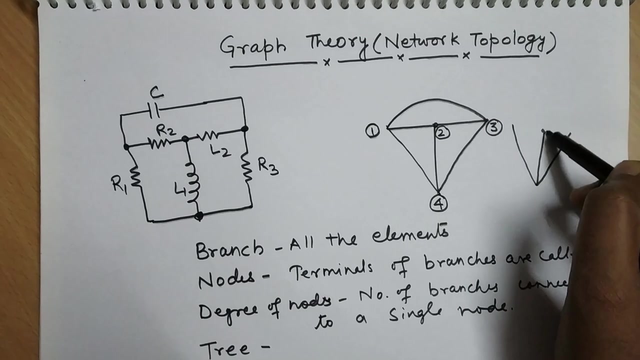 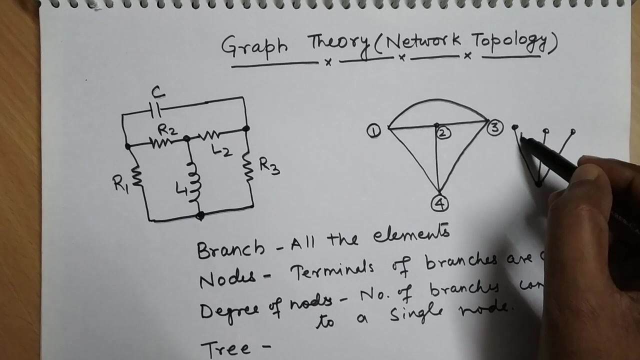 to a single node. then comes tree. it is interconnected, open set of branches which includes all the nodes of the given graph. so let us take this graph and consider a combination like this so we can see that in this combination all the nodes are covered. all the four nodes are. 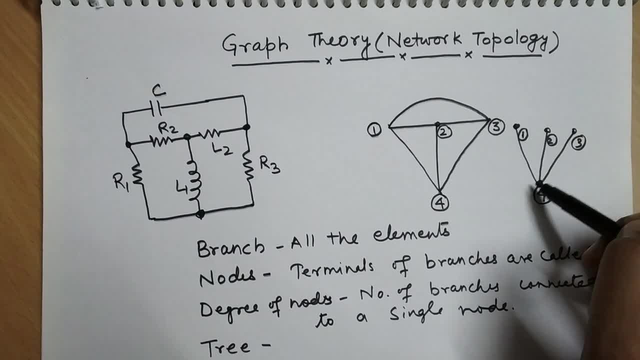 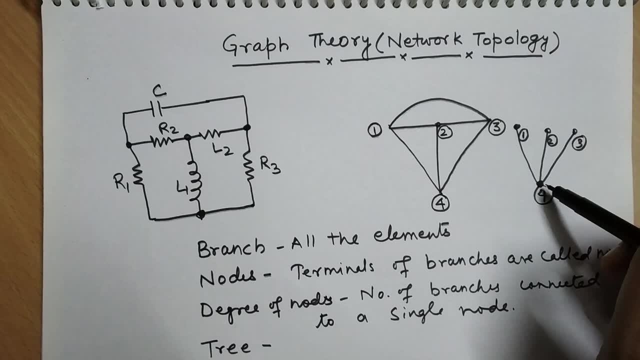 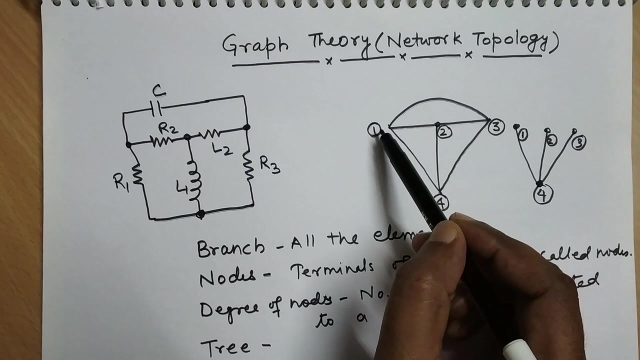 connected but there is no loop in the graph. loop means if the combination of branch makes a closed path then it is called a loop. here none of the branches makes a closed path. so these three combination of branches are called as tree. so tree can be many combination for a particular given circuit. let's say I have taken 1. 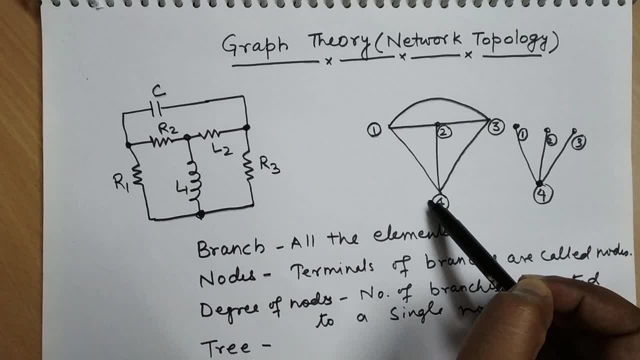 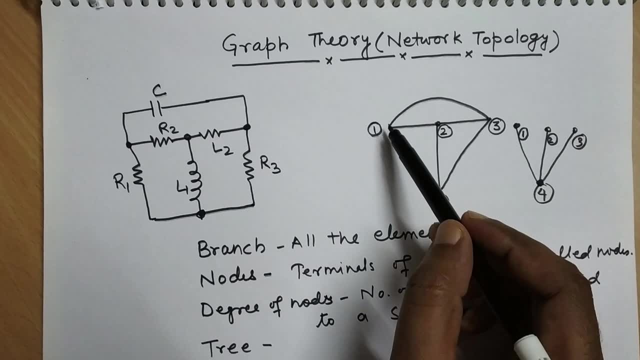 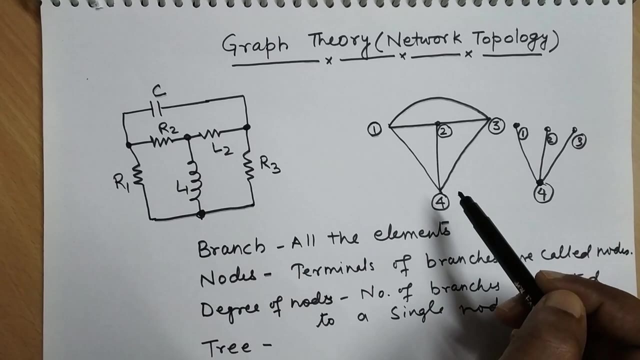 2, 4, 2, 2, 4 and 3, 2, 4. so 1, 2, 3, 4. all the nodes are covered. so 1, 2, 4 and 2, 2, 4 and 3, 2, 4 is called as a tree combination. similarly, someone would have taken 1: 2. 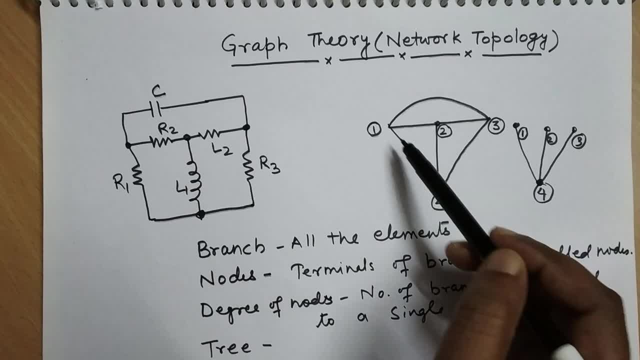 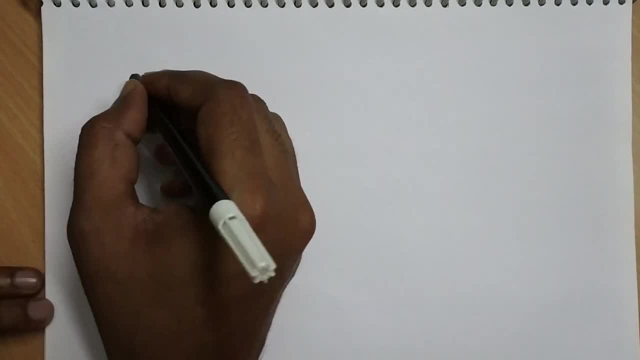 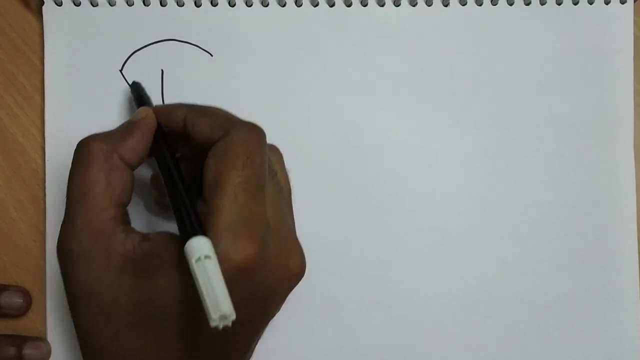 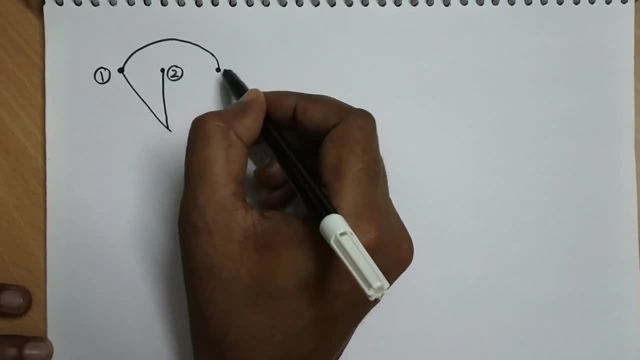 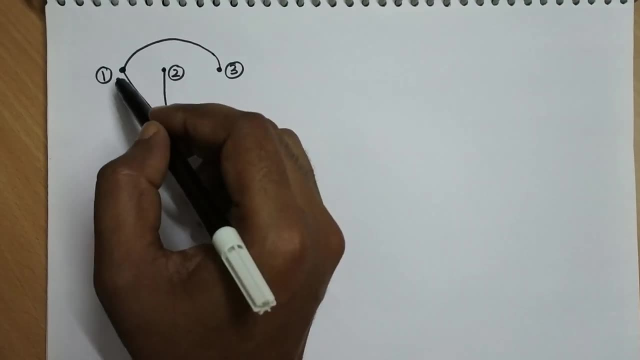 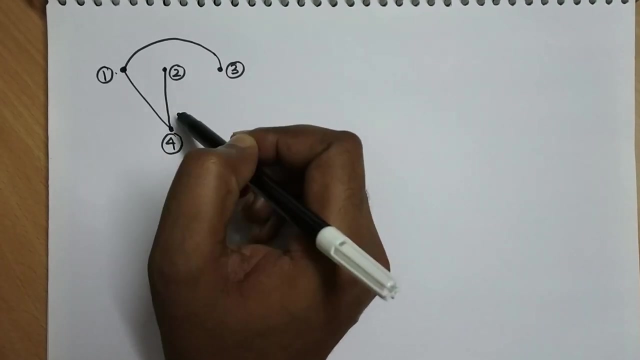 node 2, node 3 and node 4. in this case also, we can see that all the nodes are connected to a branch and connected to a branch, and connected to a branch, and none of the combination makes a loop. so this is. none of the combination makes a loop. so this is. 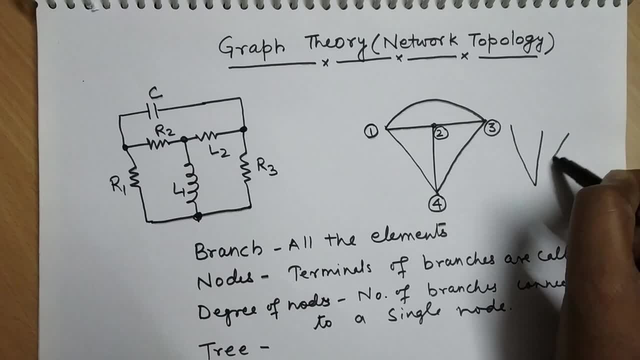 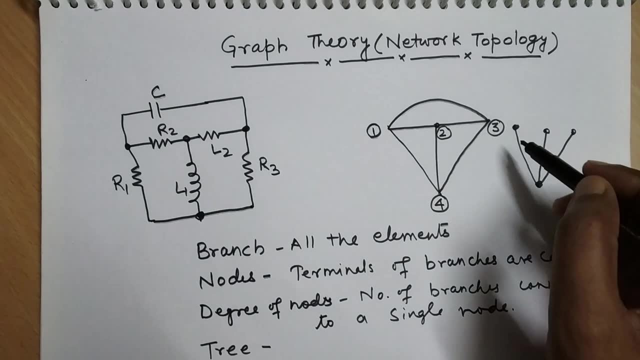 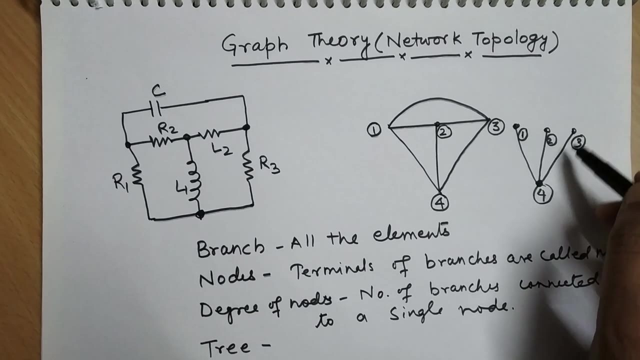 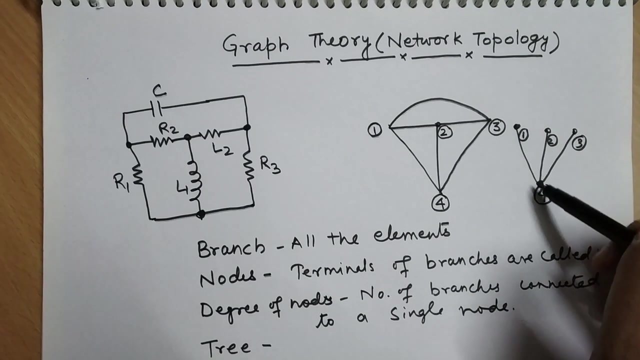 So we can see that in this combination all the nodes are covered, All the four nodes are connected, But there is no loop in the graph. Loop means if the combination of branch makes a closed path, then it is called a loop. So if the combination of branch makes a closed path, then it is called a loop. 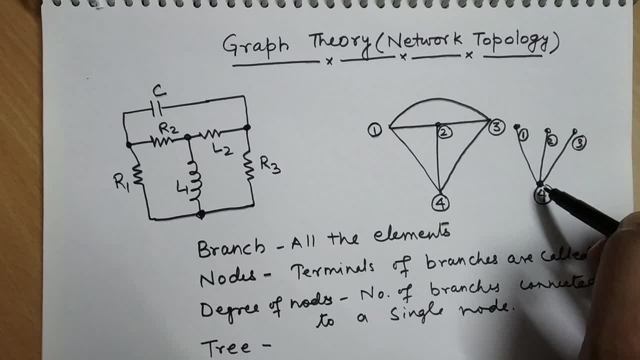 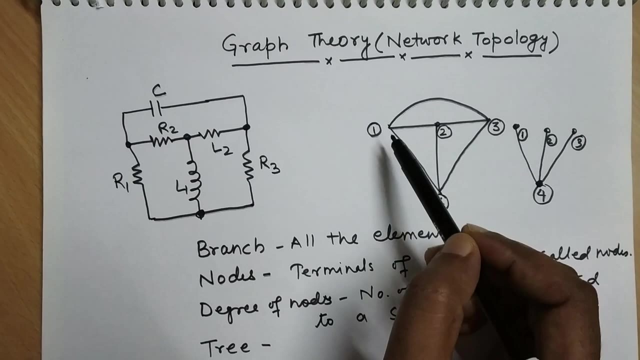 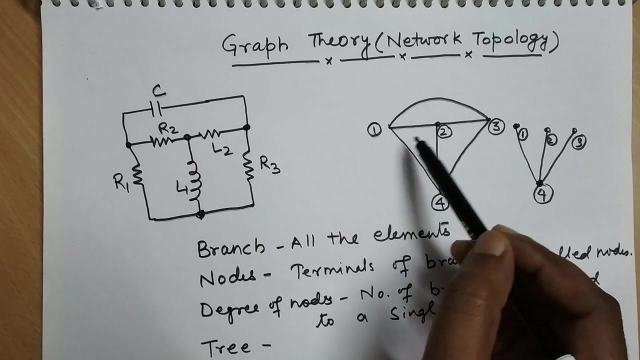 Here none of the branches makes a closed path. So these three combination of branches are called as tree. So tree can be many combination for a particular given circuit. Let us say I have taken one, two, four, two, two, four and three, two, four. So one, two, three, four, all the nodes are. 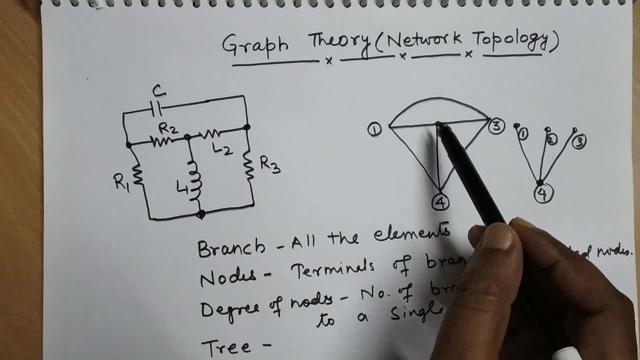 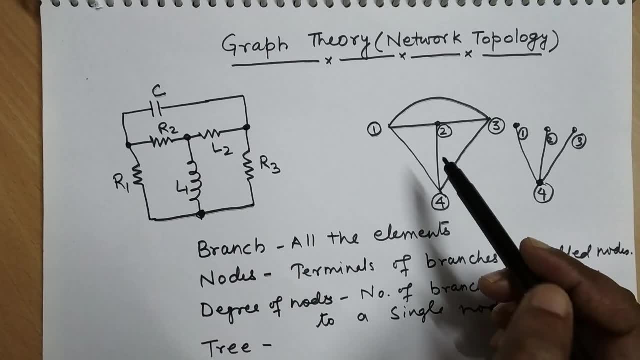 covered. So one, two, four and two two, four and three, two, four is called as a tree combination. Similarly, someone would have taken one, two, three, two two, four and one two, four. 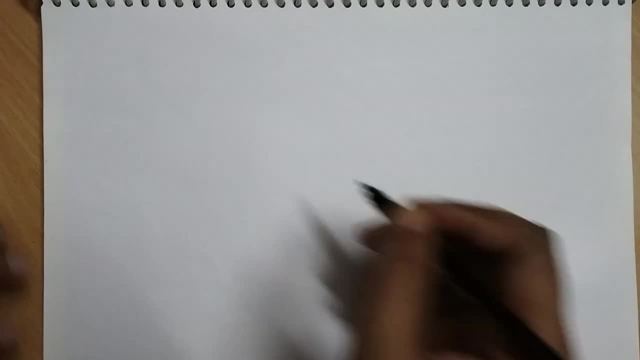 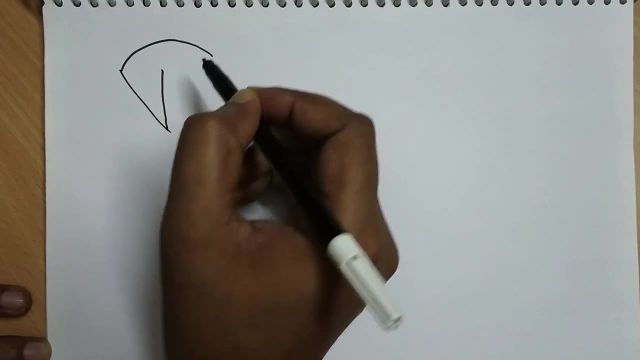 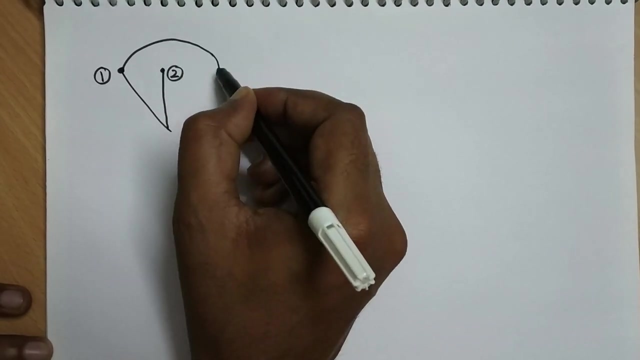 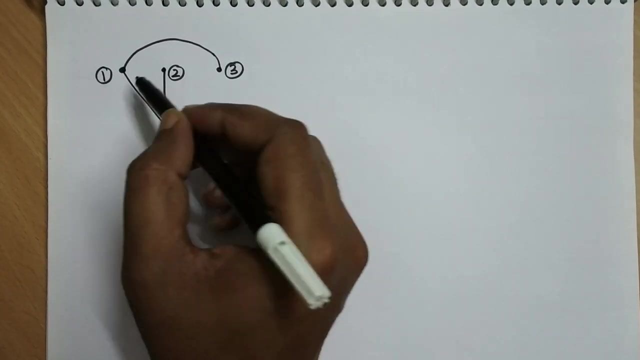 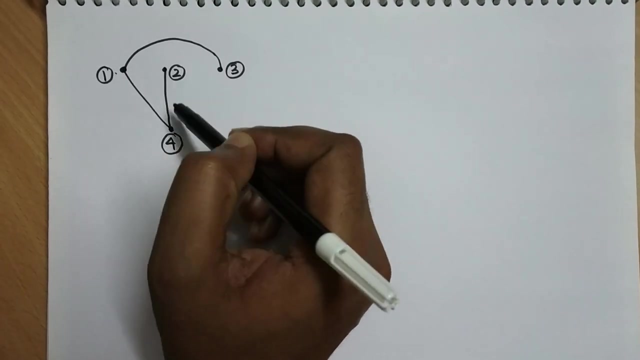 So let us take that. So another tree combination may be something like this, But this is node 2, node 3 and node 4.. In this case also, we can see that all the nodes are connected to a branch and none of the combination makes a loop. So this is also. 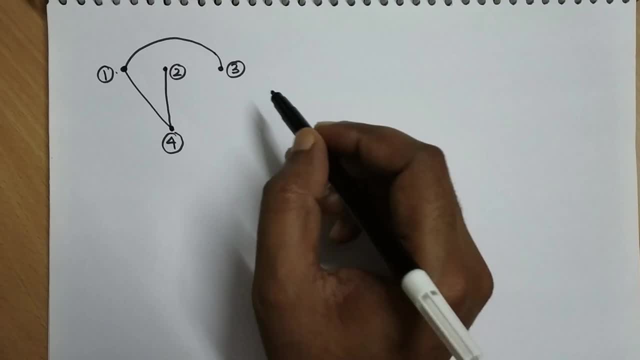 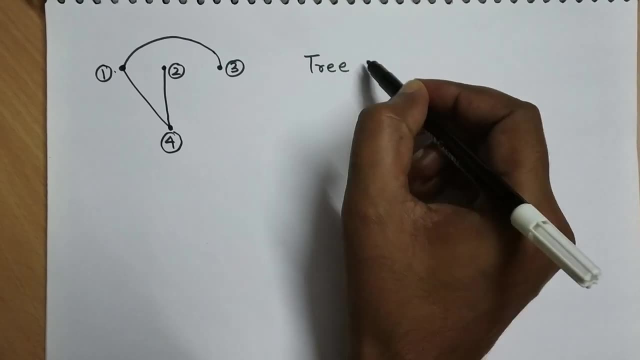 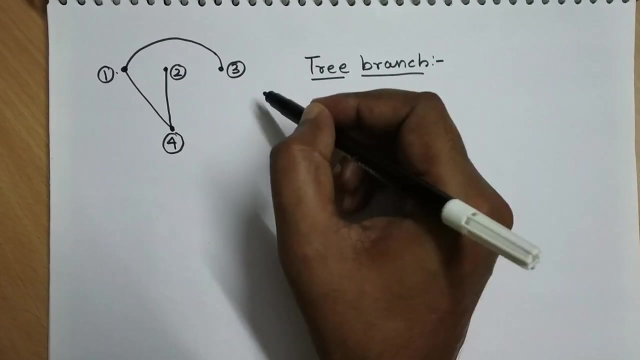 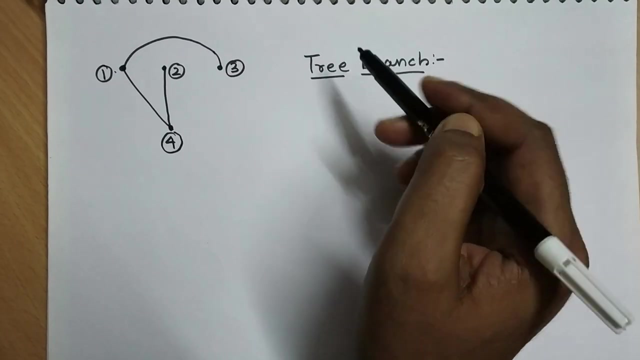 one of the combination of tree. So there are many combination of tree is possible. Now next comes tree branch. So, as name says, tree branch. So for a given tree all the branch are called as a tree branch, If I assume that this is branch number 1,. 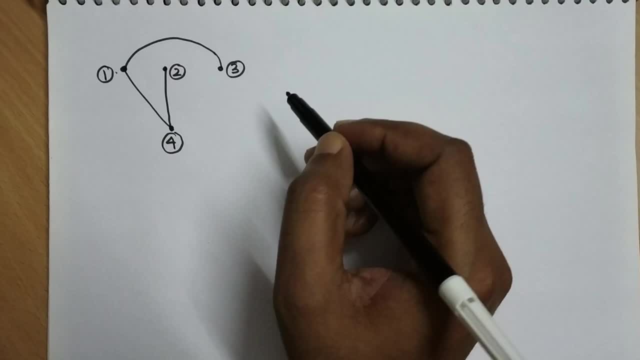 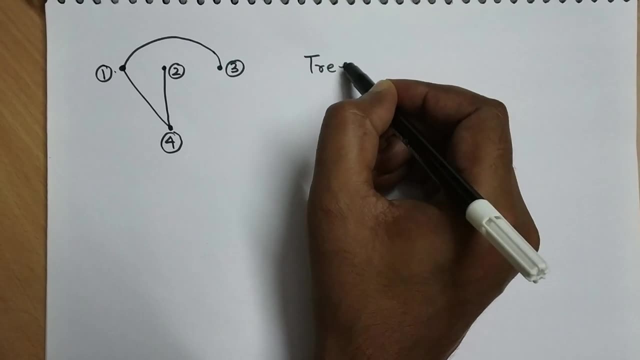 none of the combination makes a loop. so this is also one of the combination of, also one of the combination of, also one of the combination of tree. so there are many combination of tree is tree. so there are many combination of tree is tree, so there are many combination of tree is possible. now next comes tree. 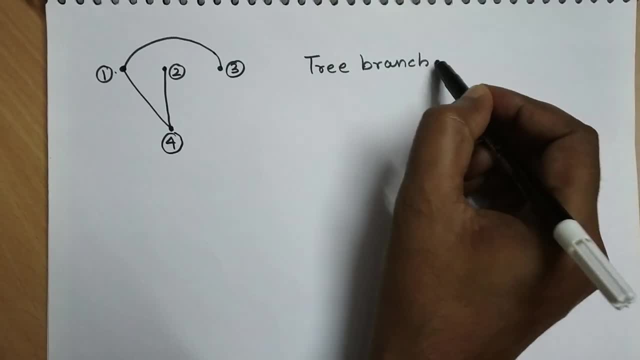 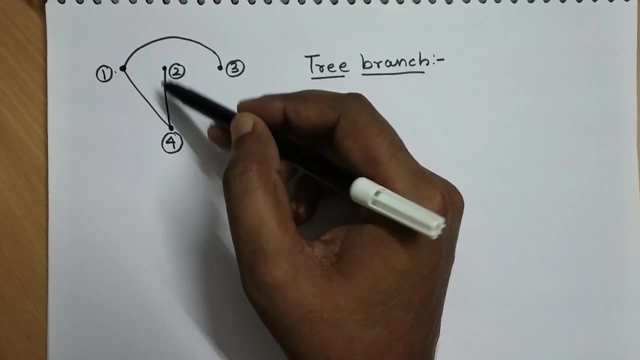 possible now. next comes tree. possible now. next comes tree branch. so as name says tree branch, so for a given branch, so as name says tree branch, so for a given branch, so for a given tree, all the branch are called as a tree branch. if I tree, all the branch are called as a tree branch if I 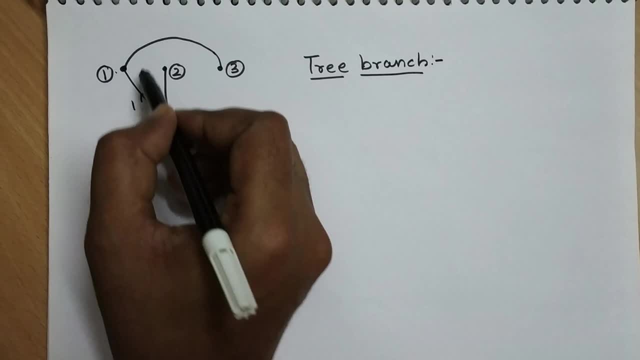 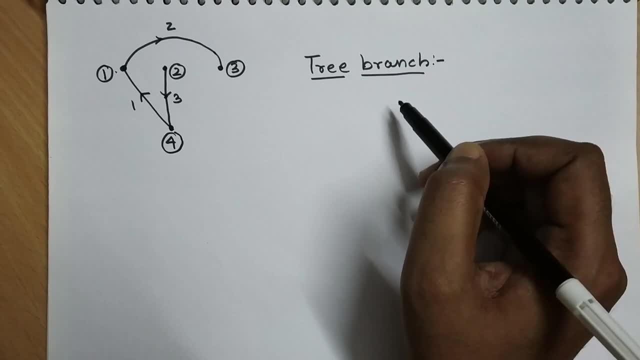 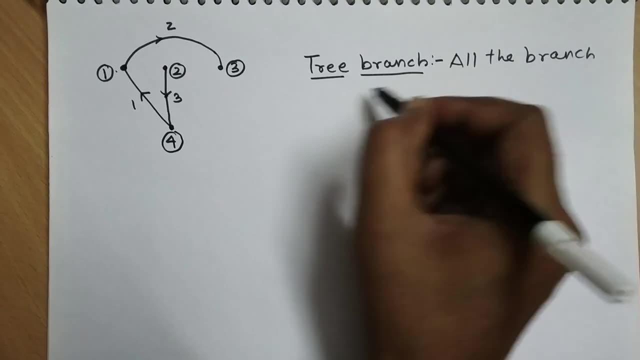 number 2, branch number 3, then these number 2, branch number 3, then these three branches are called as a tree. three branches are called as a tree. three branches are called as a tree branch. so all the branch of tree is branch. so all the branch of tree is. 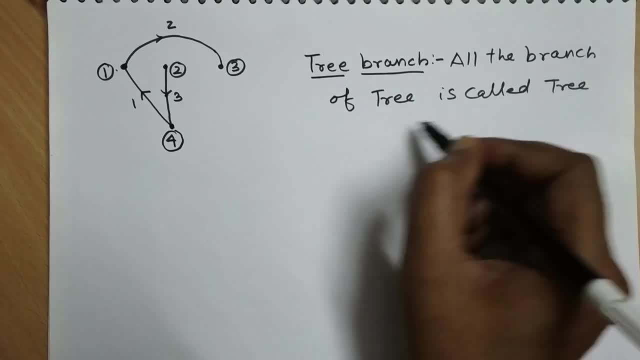 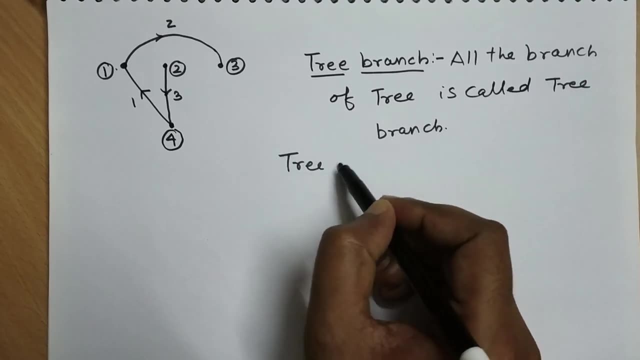 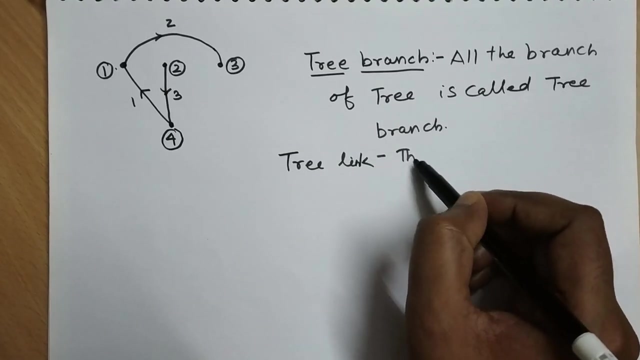 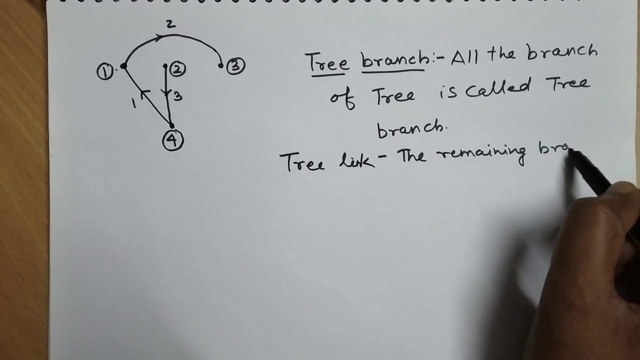 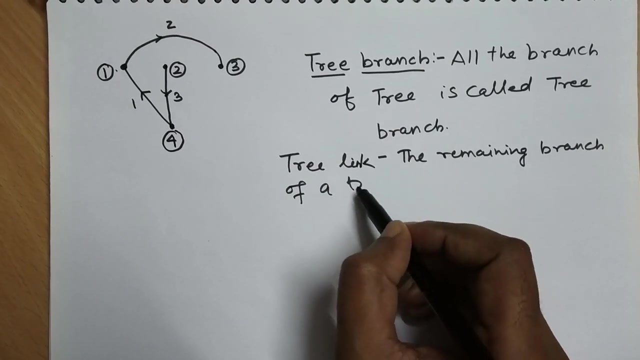 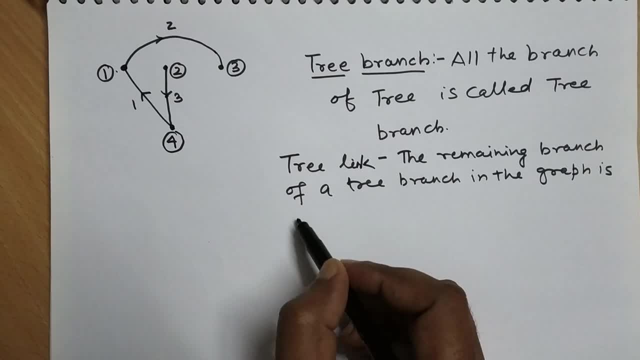 so the remaining branch of a tree branch in the graph. so the remaining branch of a tree branch in the graph. so the remaining branch of a tree branch in the graph is called as link. so for example in this is called as link. so for example in this: 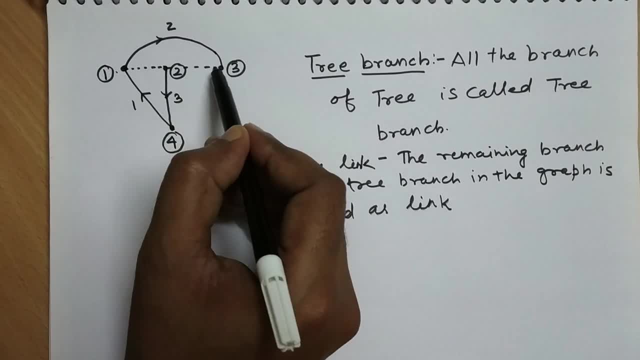 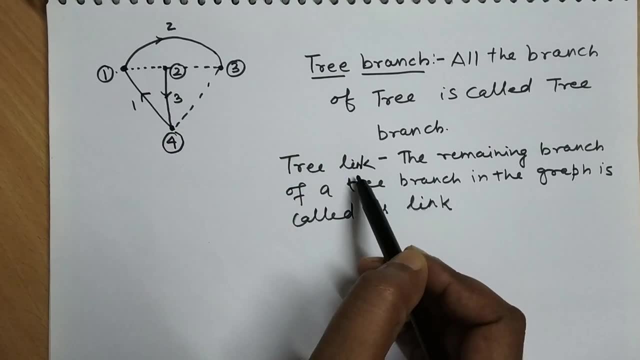 is called as link. so, for example, in this case, these are the remaining branches, so case, these are the remaining branches, so case, these are the remaining branches. so these three branches are called as tree, these three branches are called as tree, these three branches are called as tree link. then, as I have discussed the loop, 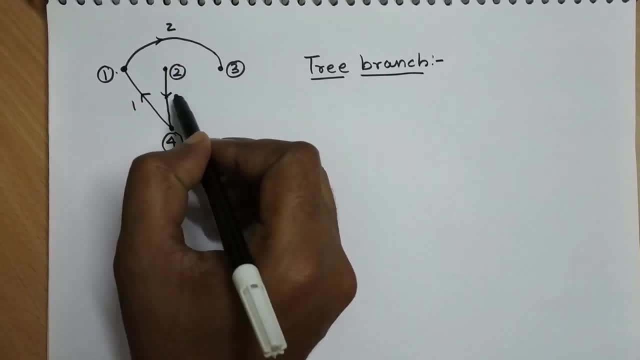 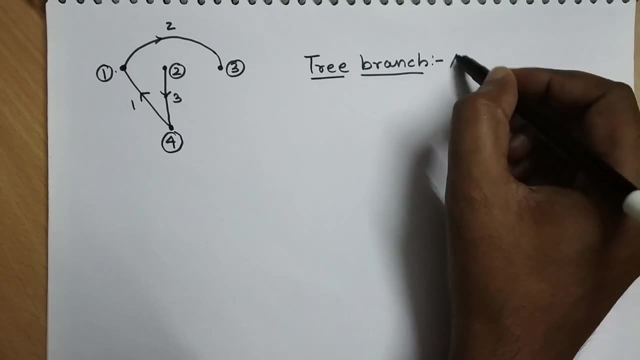 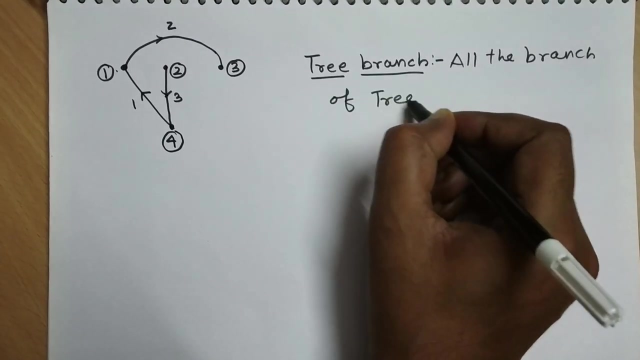 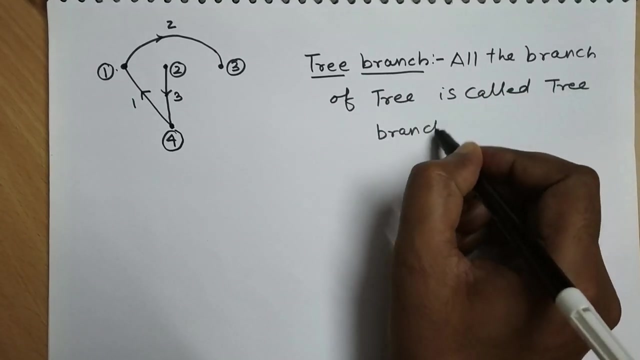 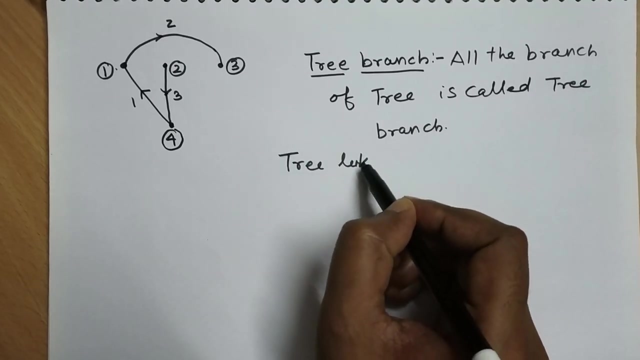 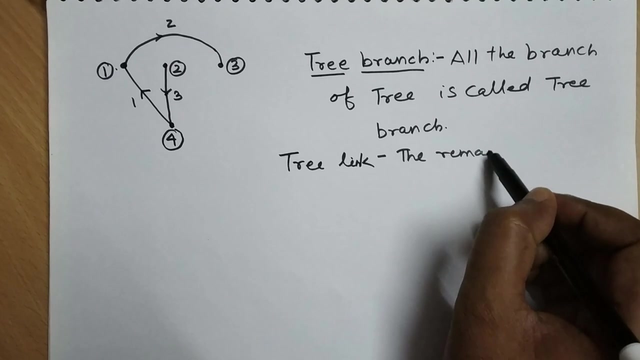 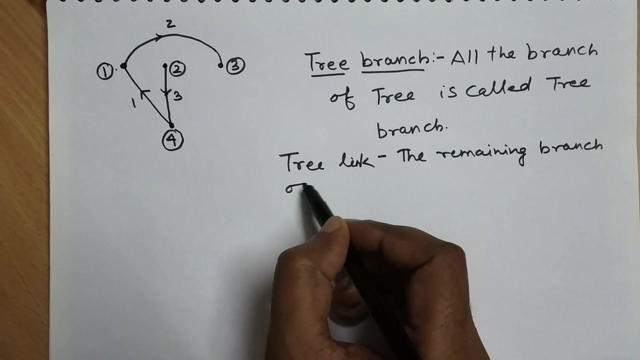 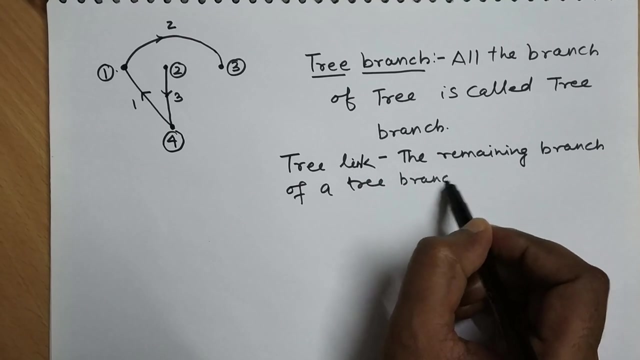 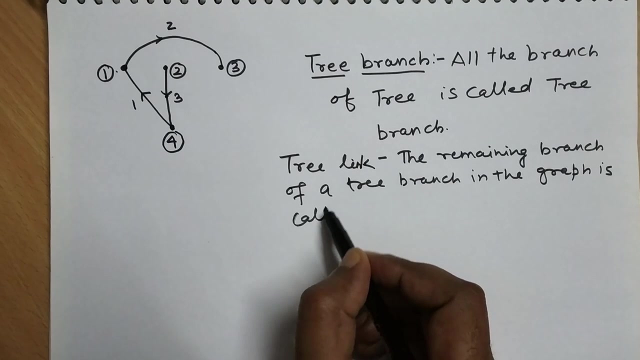 branch number 2, branch number 3. then these three branches are called as a tree branch, So all the branch of tree is called tree branch, Then tree link, So the remaining branch of a tree branch in the graph is called as link. So for example in: 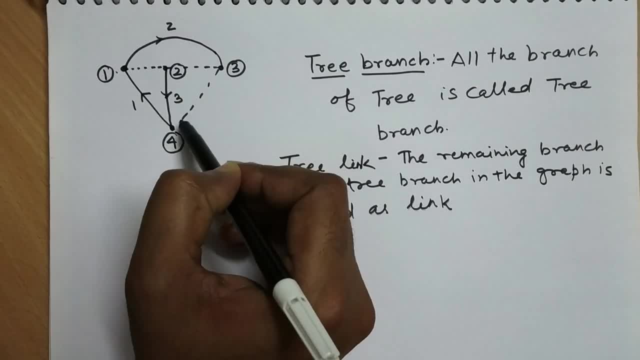 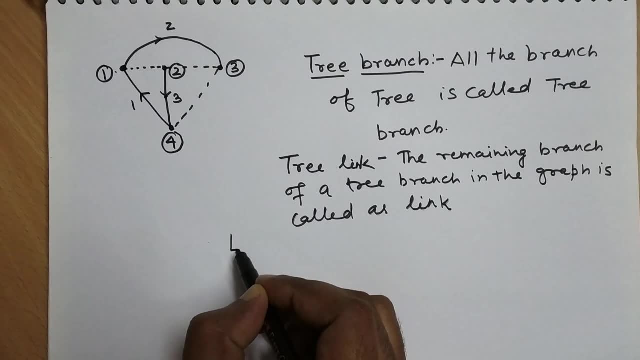 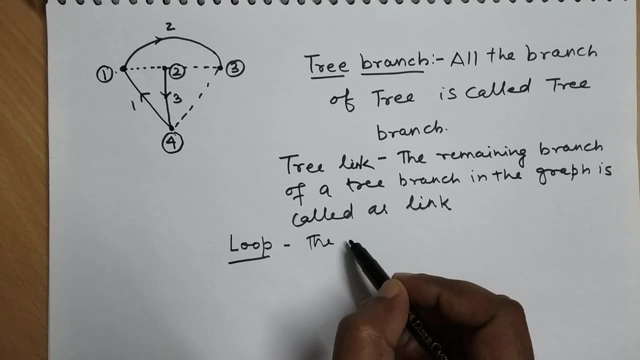 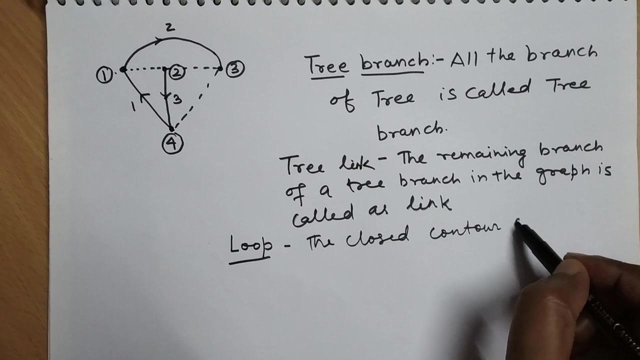 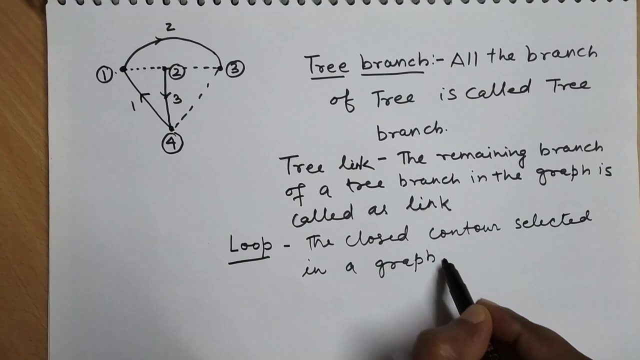 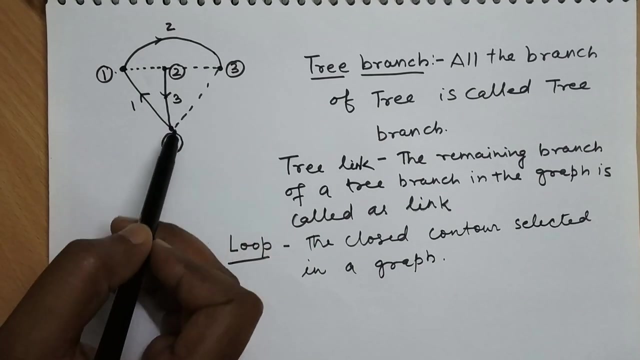 the graph. these are the remaining branches. So these three branches are called as tree link. Then, as I have discussed, the loop Loop is the closed contour selected in a graph. So, for example, if I take from 2 to 3, 3 to 4 and 4 to 2, this will become a loop. Similarly, 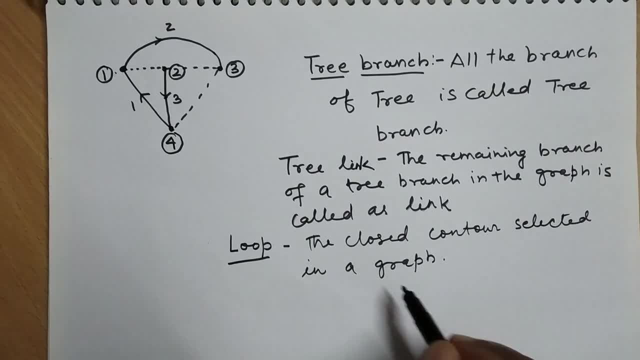 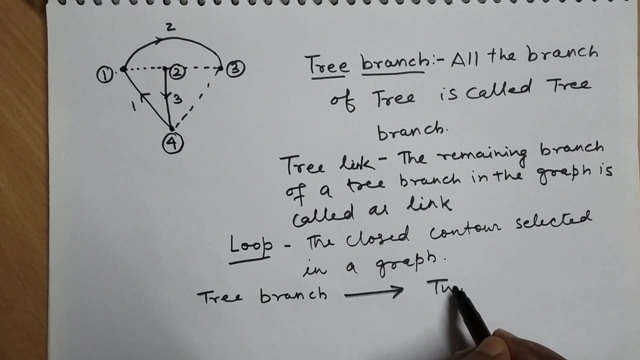 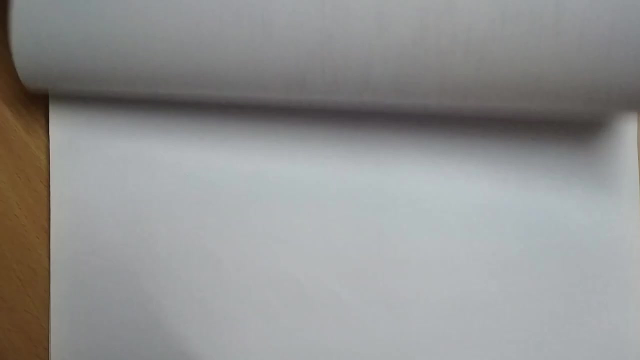 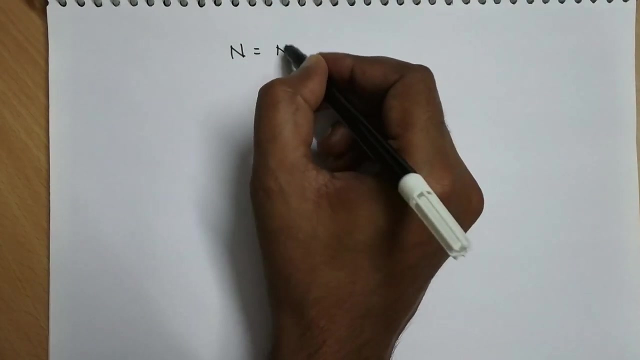 if we take 1 to 2, 2 to 4 and 4 to 1, that will also become a loop. Now the tree branch is also known as twig. Now we will see the relation between twigs and links. So let us say n is equal to number. 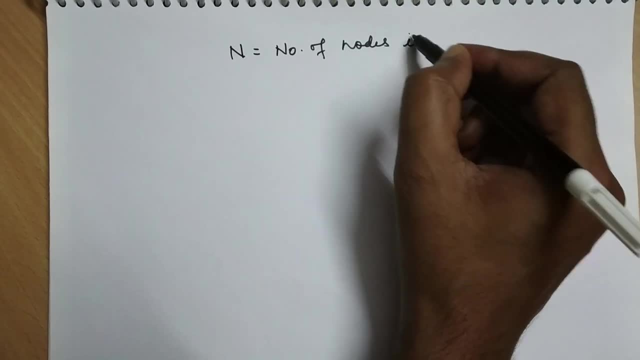 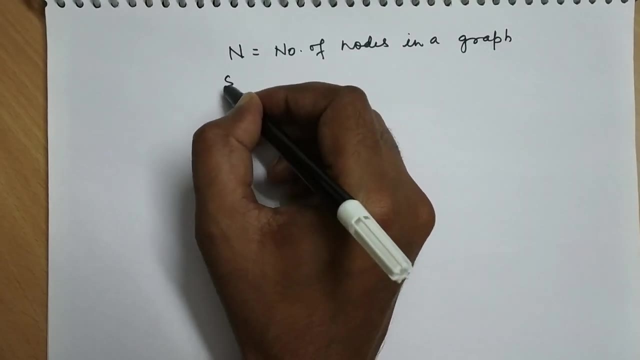 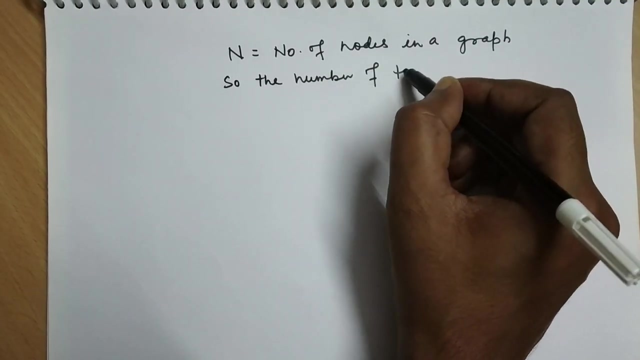 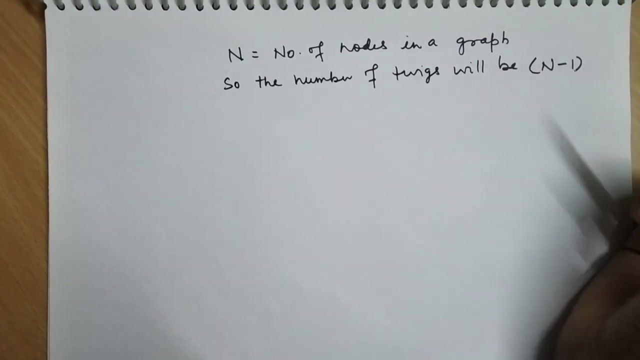 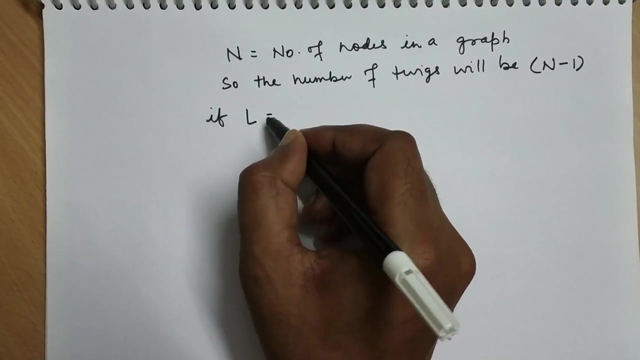 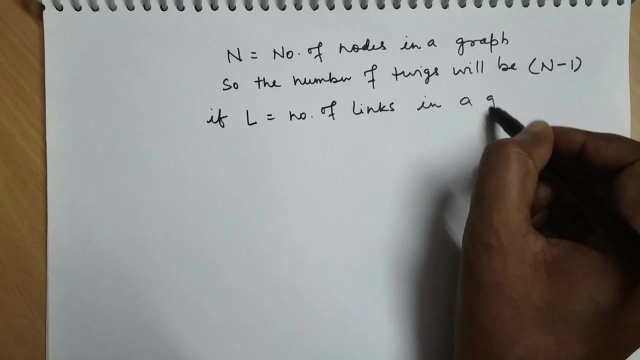 of nodes in a graph. So the number of twigs will be n minus 1.. And if l represents the number of links in a graph, Now we will see the relation between twigs and links. So let us say n is equal to number of nodes in a graph. 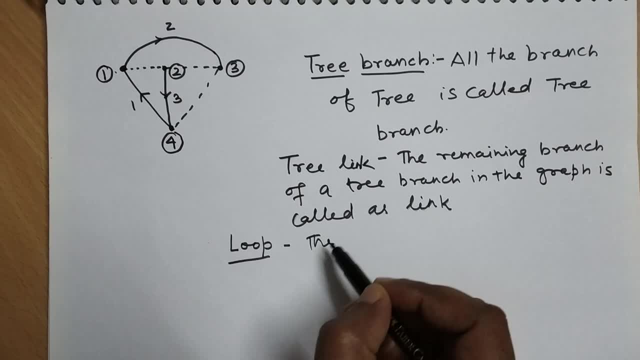 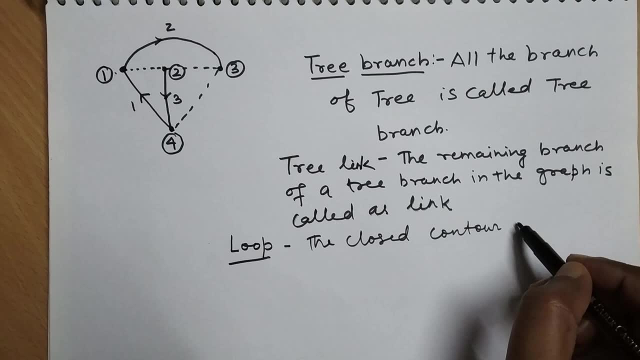 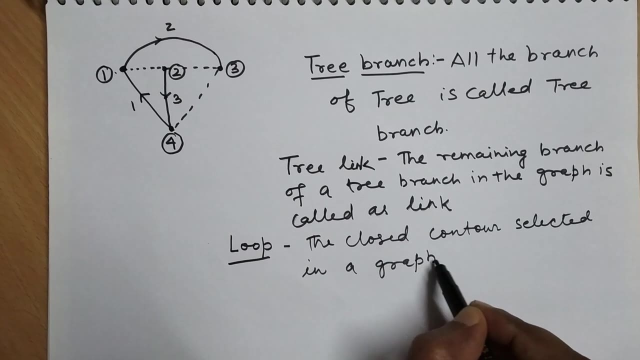 link, then, as I have discussed the loop link, then, as I have discussed the loop loop, is the closed loop, is the closed loop is the closed contour selected in a graph. so, for example, if I contour selected in a graph. so, for example, if I contour selected in a graph. so, for example, if I take from 2 to 3, 3 to 4 and 4 to 2, take from 2 to 3, 3 to 4 and 4 to 2. take from 2 to 3, 3 to 4 and 4 to 2. this will become a loop, similarly if we. this will become a loop, similarly if we. 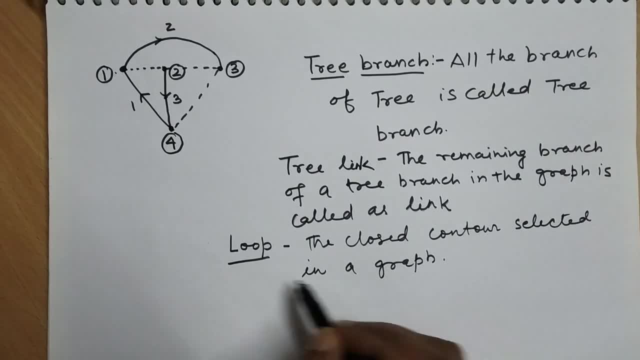 this will become a loop. similarly, if we take 1 to 2, 2 to 4 and 4 to 1, that will take 1 to 2, 2 to 4 and 4 to 1. that will take 1 to 2, 2 to 4 and 4 to 1. that will also become a loop. now, the tree branch. 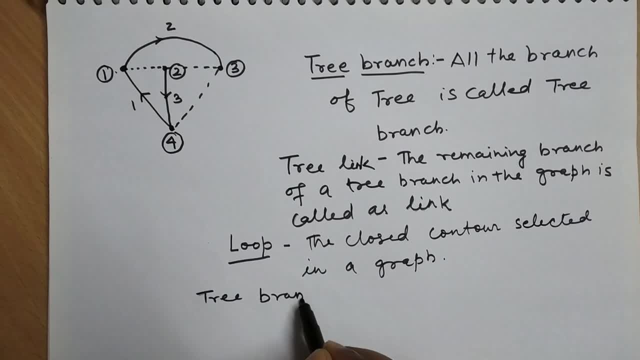 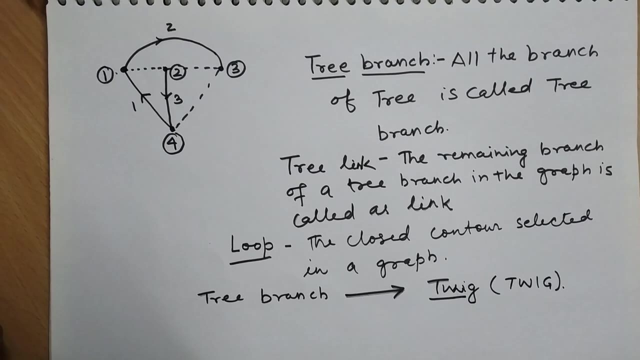 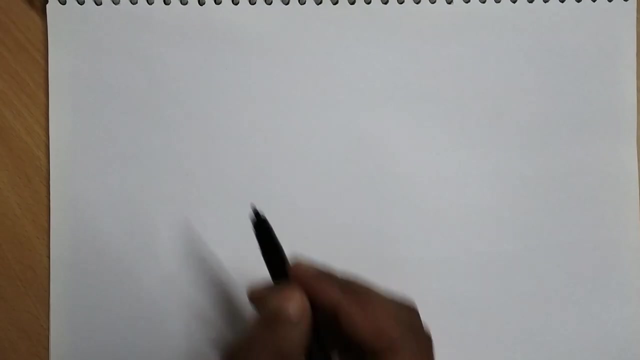 also become a loop. now the tree branch also become a loop. now the tree branch is also known as Twig- now we will see is also known as Twig- now we will see is also known as Twig. now we will see the relation between twigs and links. so 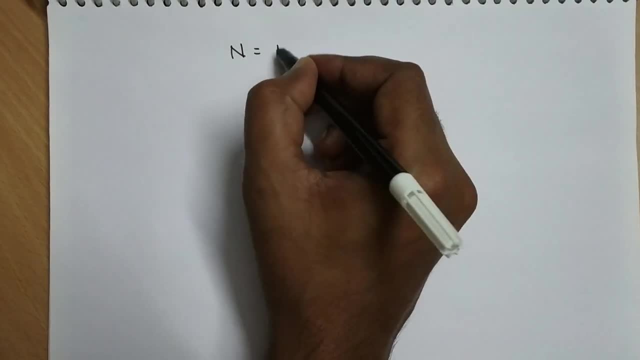 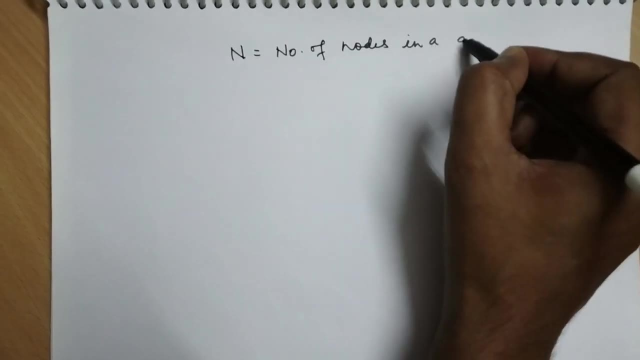 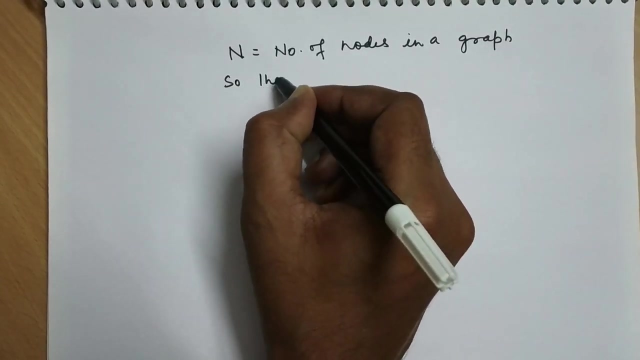 the relation between twigs and links. so the relation between twigs and links. so let us say n is equal to, let us say n is equal to. let us say n is equal to number of nodes in a graph. so the number of nodes in a graph, so the 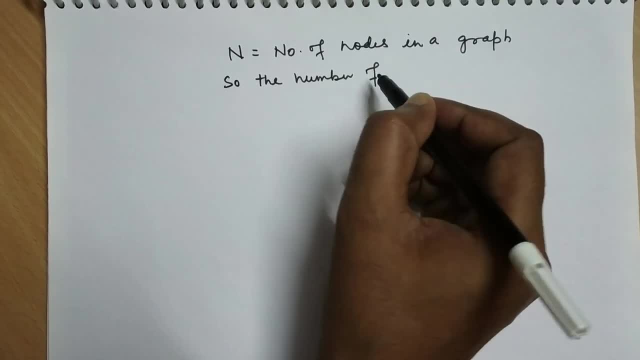 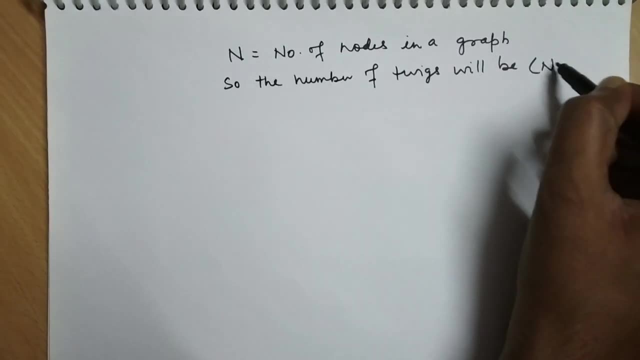 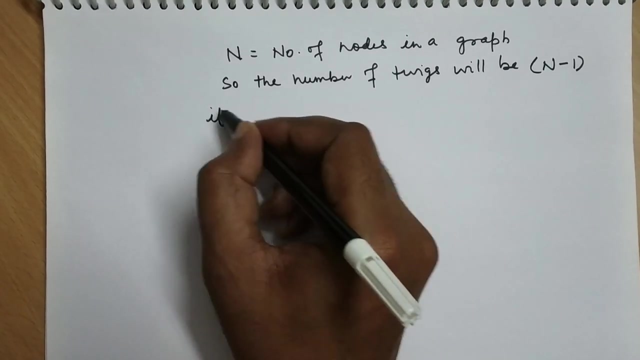 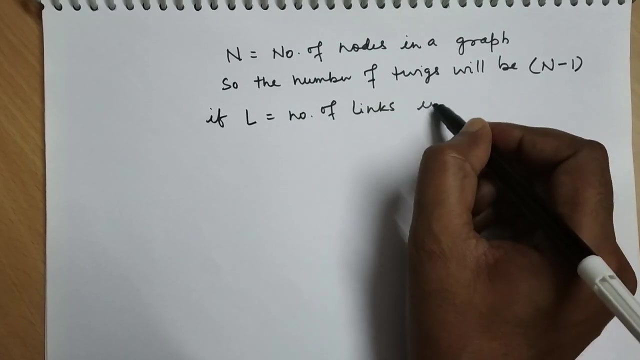 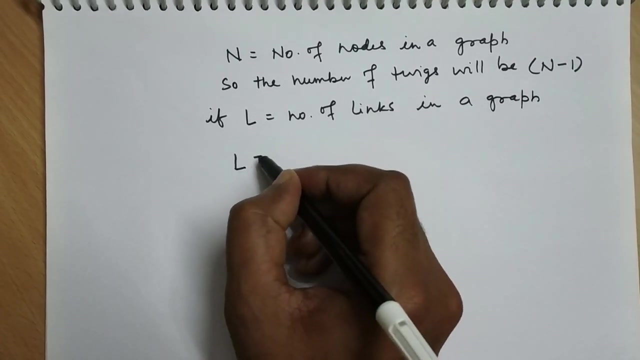 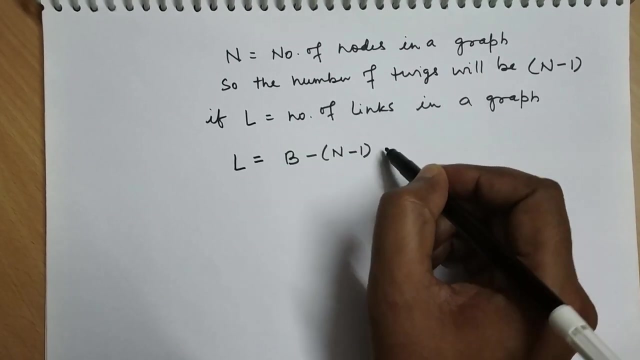 number of nodes in a graph. so the number of pigs will be n minus 1 and number of pigs will be n minus 1. and if L represents the number of links in, if L represents the number of links in, if L represents the number of links in a graph, then L equal to B minus n minus 1. 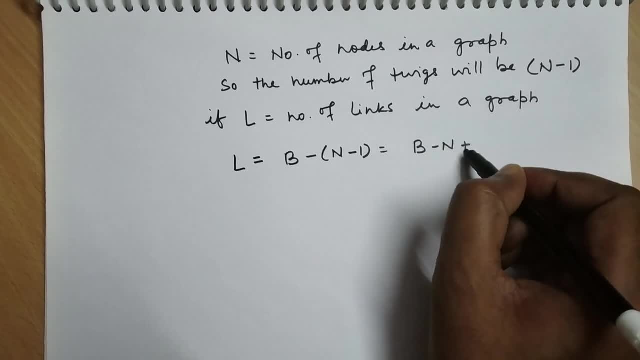 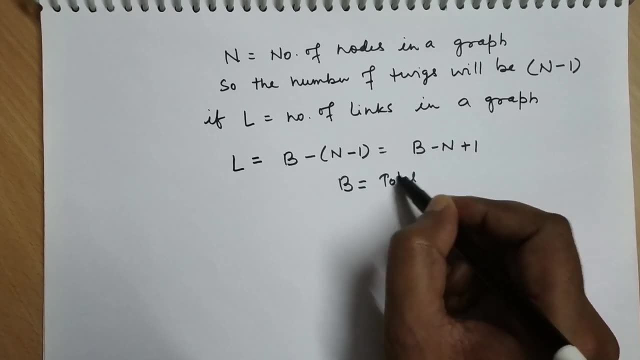 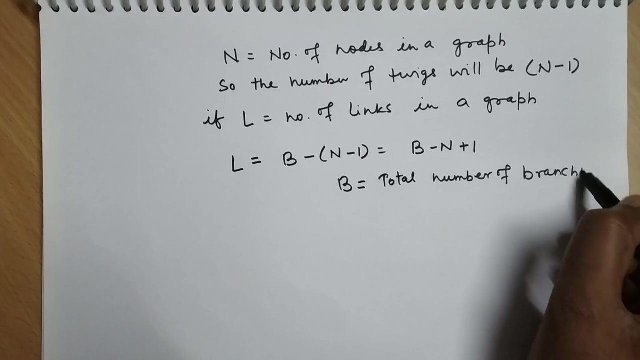 a graph then L equal to B minus n minus 1. a graph then: L equal to B minus n minus 1. which is equal to B minus n plus 1. where which is equal to B minus n plus 1. where which is equal to B minus n minus 1. where B is total number of branch in the graph. 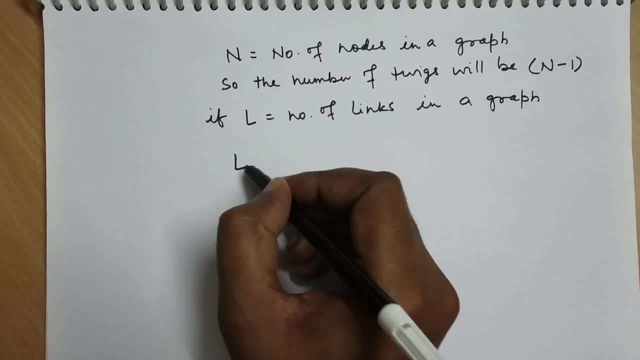 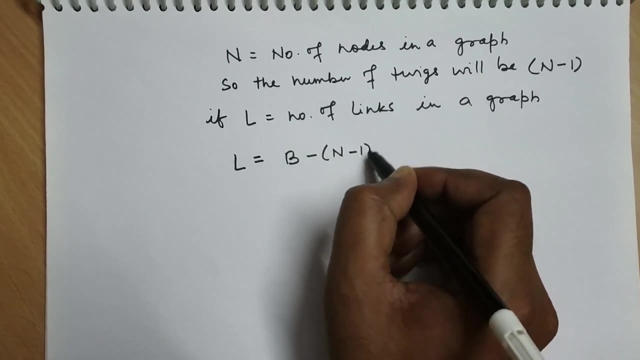 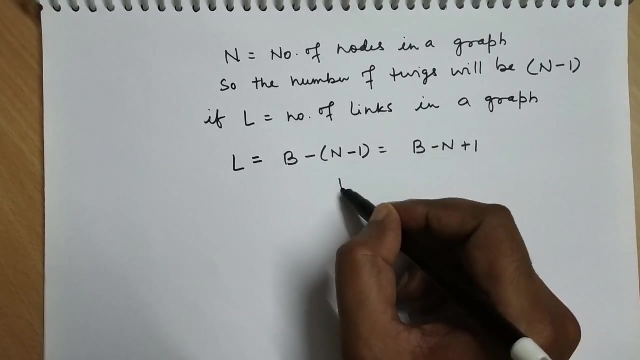 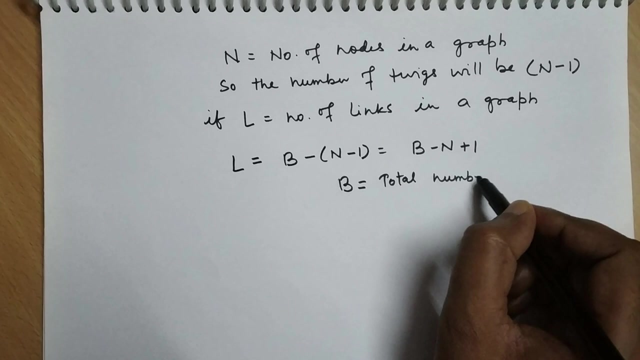 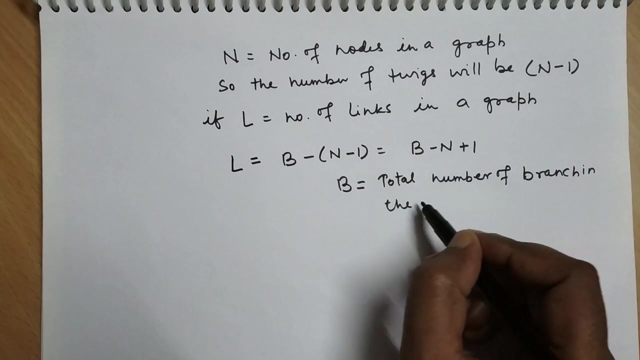 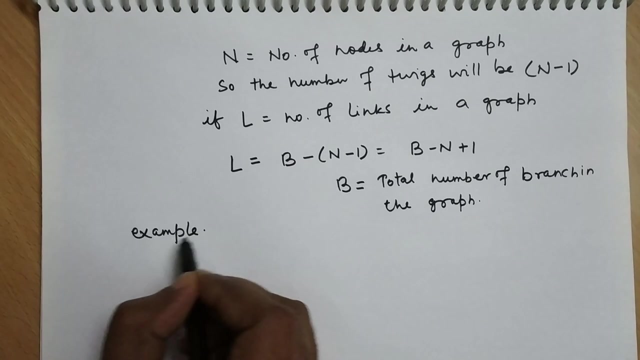 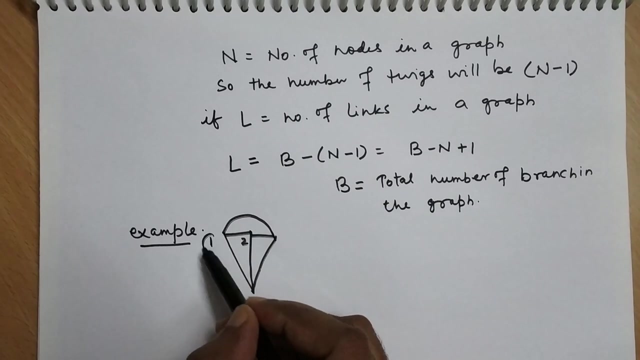 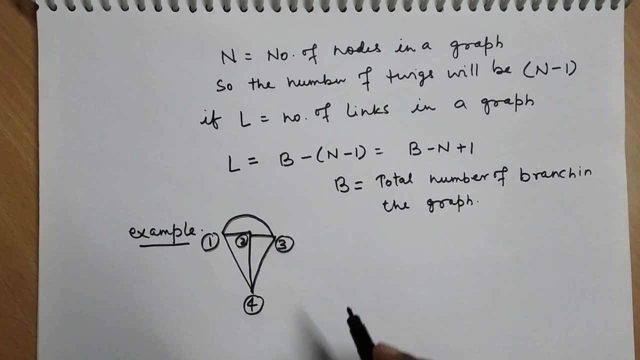 Then l equal to b minus n minus 1, which is equal to b minus n plus 1, where b is total number of branch In the graph. For example, if I consider the same graph, 1, 2, these are the nodes 2, 3, 4.. So in this particular graph, n, which is number of nodes equal to 4.. 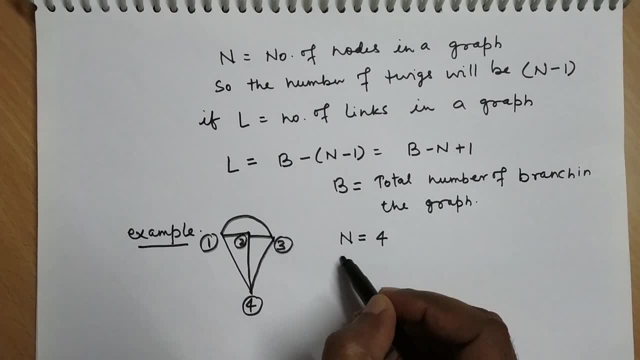 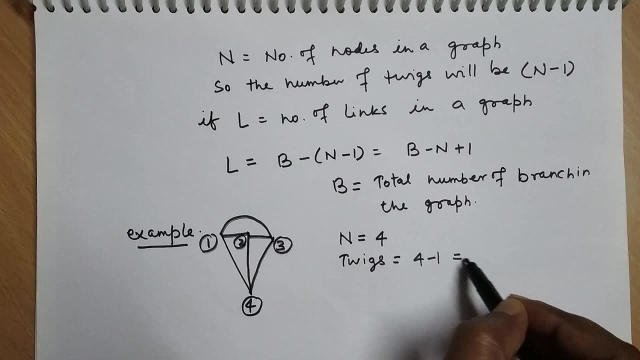 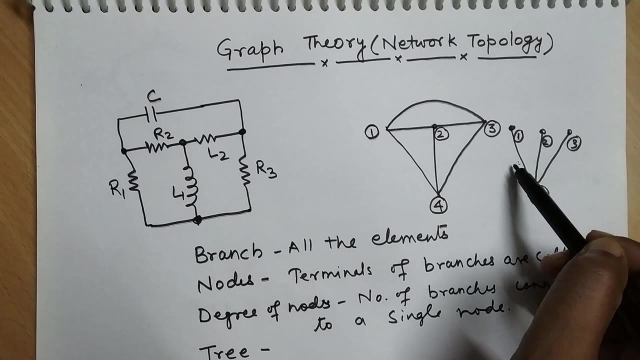 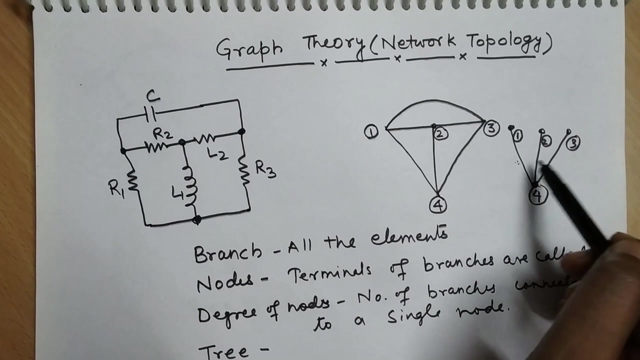 So the number of twigs: number of twigs equal to 4 minus 1, which is equal to 3.. As we have seen for the tree formed using this graph for the same example, by considering a different combination of tree branches, there are 3 tree branches taken to form a tree. 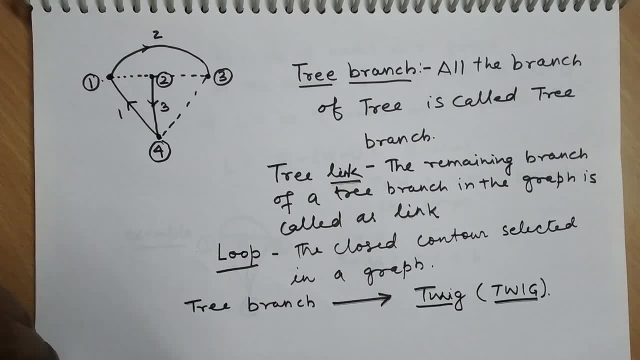 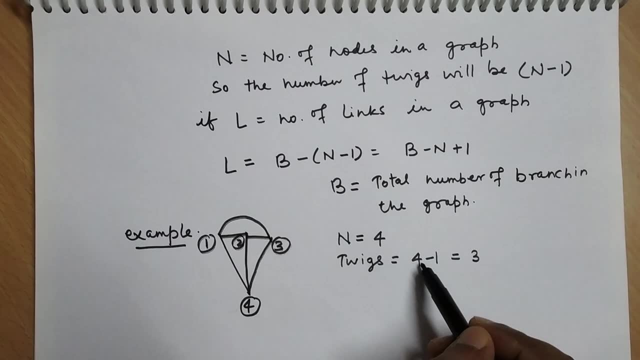 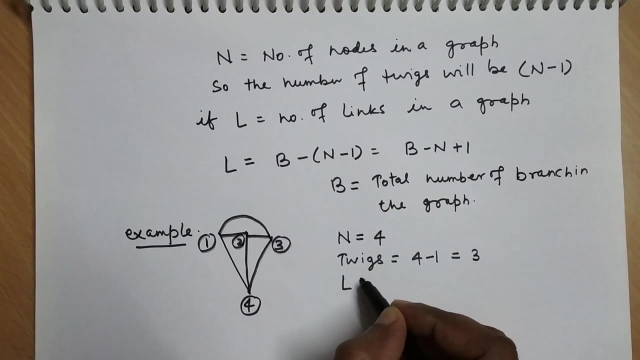 In this case also, 3 branches are considered to form a tree. So the number of tree branches, or number of twigs, equal to 4 minus 1, equal to 3.. Now l, which is number of links in a given graph, So the remaining branches are called as links. So there are total of 6 branches in the graph. So 3 branches are twigs, So remaining 3 branches will be links. 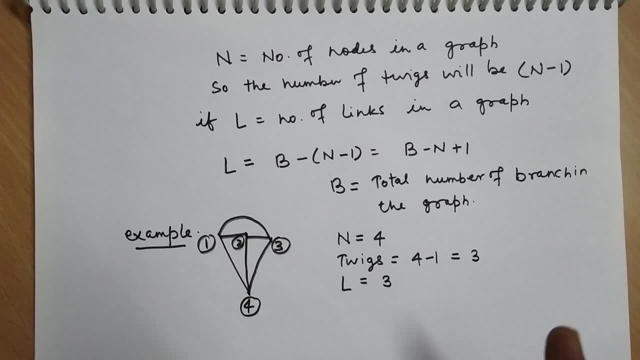 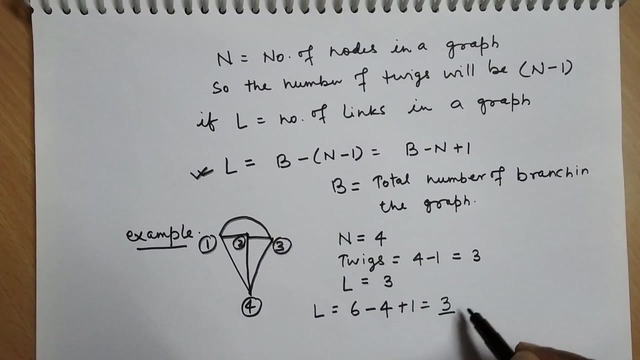 So l equal to 3.. So now we can get this relation, which is l to find number of links. So l equal to total number of branch, 6 minus number of nodes, that is 4 plus 1.. 6 minus 4 plus 1 is 3.. So there, 3 is number of links. 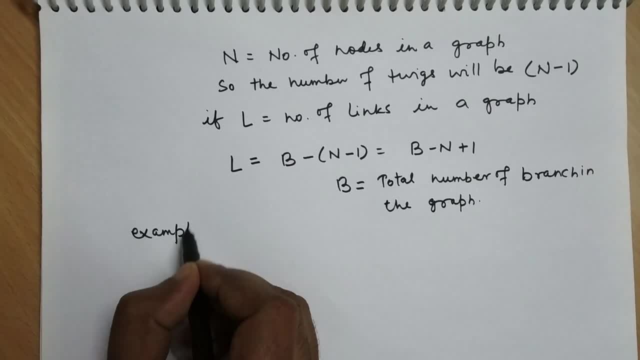 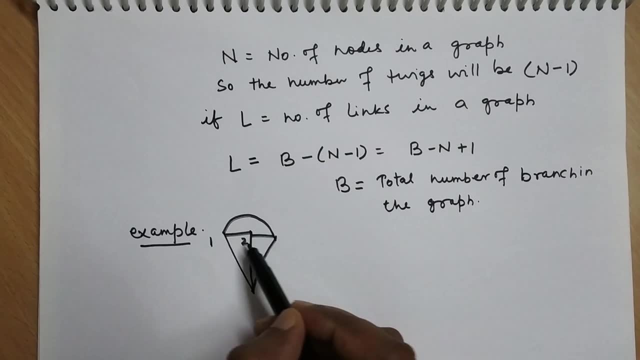 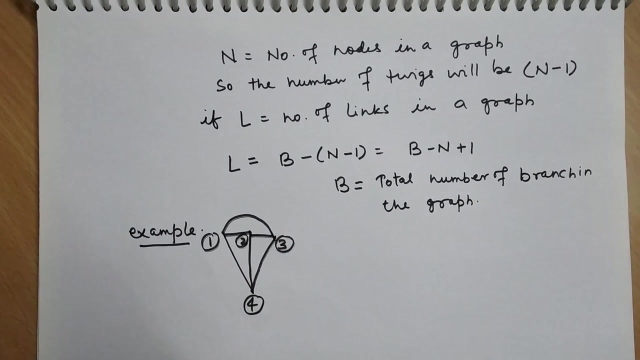 B is total number of branch in the graph. B is total number of branch in the graph. for example, if I consider the same graph, for example, if I consider the same graph, for example, if I consider the same graph, 1, 2, these are the nodes 2, 3, 4. so in this, 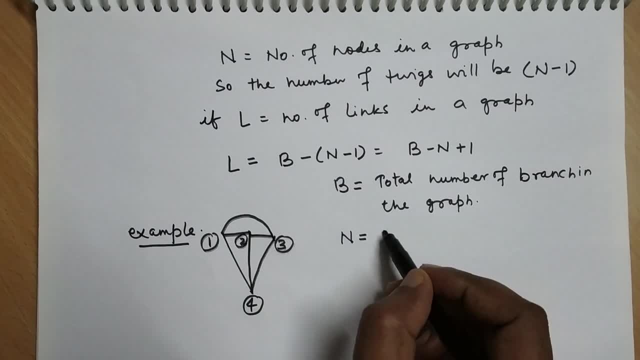 1, 2, these are the nodes 2, 3, 4. so in this 1, 2, these are the nodes 2, 3, 4. so in this particular graph n, which is number of particular graph n, which is number of particular graph n, which is number of nodes equal to 4, so the number of tweaks: 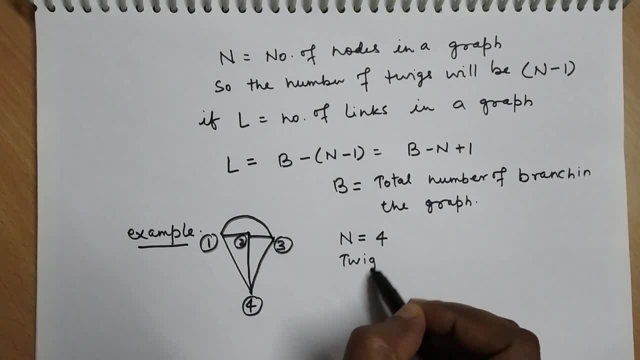 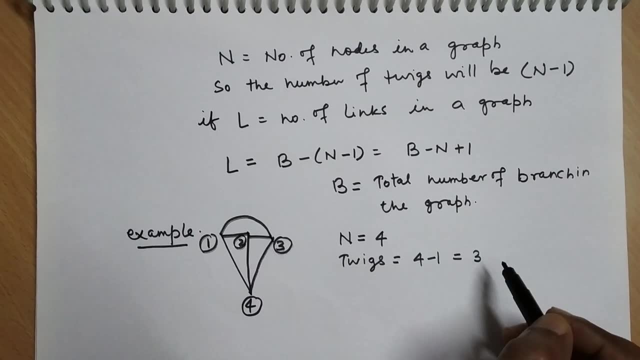 nodes equal to 4. so the number of tweaks: nodes equal to 4. so the number of tweaks: number of tweaks equal to 4 minus 1. number of tweaks: number of tweaks equal to 4 minus 1. number of tweaks: number of tweaks equal to 4 minus 1, which is equal to 3, as we have seen. 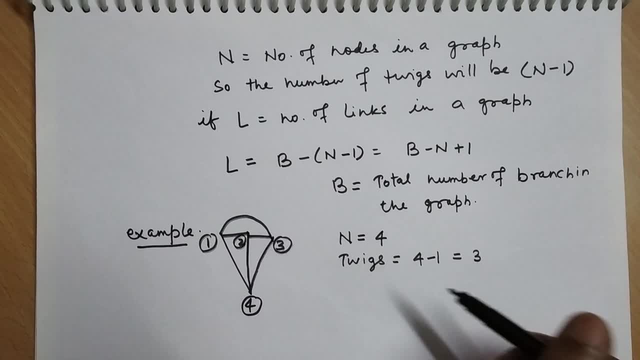 which is equal to 3, as we have seen. which is equal to 3, as we have seen, for the tree formed. using this graph for: for the tree formed. using this graph for: for the tree formed. using this graph for the same example, by considering a. the same example by considering a: 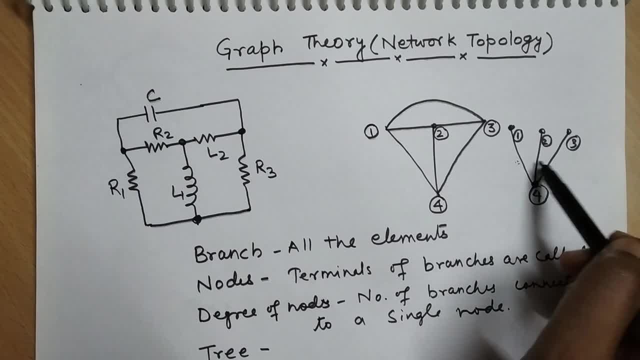 the same example by considering a different combination of tree branches, different combination of tree branches, different combination of tree branches. there are three tree branches taken to. there are three tree branches taken to. there are three tree branches taken to form a tree. in this case, also three. form a tree: in this case, also three. 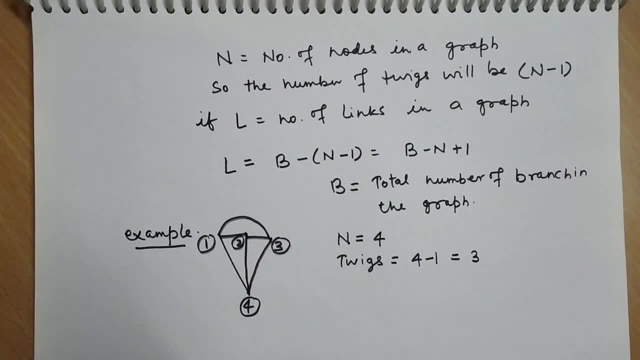 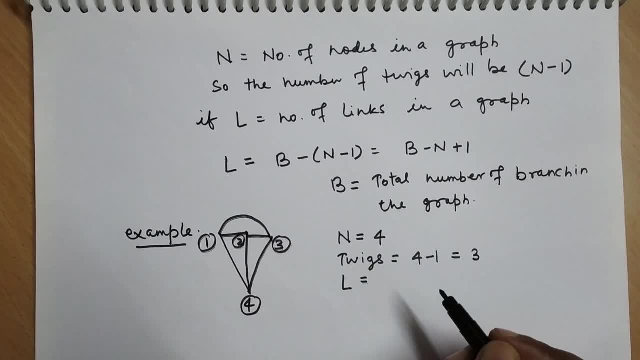 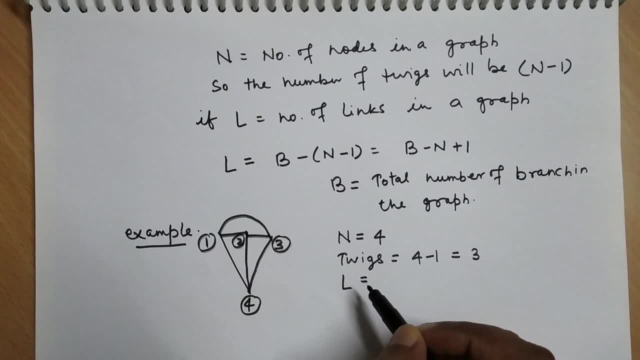 now L, which is number of links in a given graph. so the remaining branches are graph. so the remaining branches are graph. so the remaining branches are called as links. so there are total of called as links. so there are total of called as links. so there are total of six branches in the graph, so three. 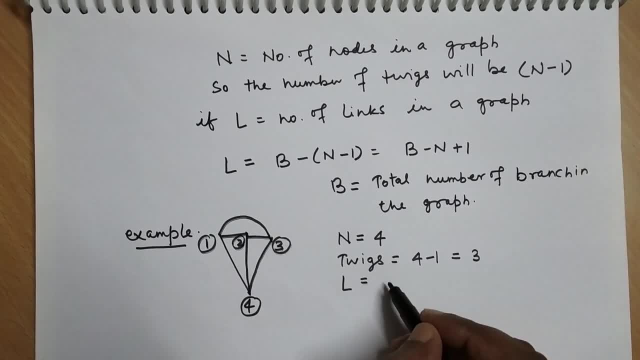 six branches in the graph, so three. six branches in the graph, so three branches are twigs. so remaining three branches are twigs. so remaining three branches are twigs. so remaining three branches will be links, so L equal to 3 branches will be links, so L equal to 3. 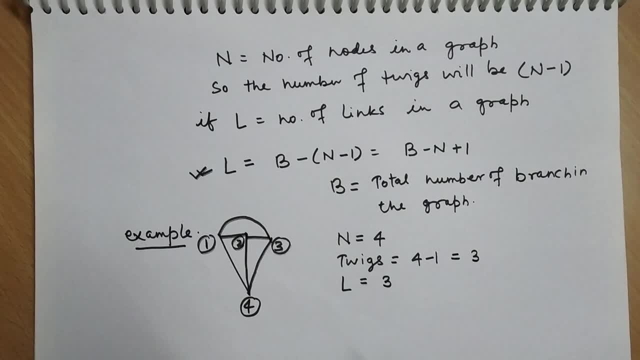 branches will be links, so L equal to 3. so now we can get this relation, which is so now we can get this relation, which is: so now we can get this relation, which is: L to find number of links. L to find number of links. L to find number of links: L equal to total number of branch 6. 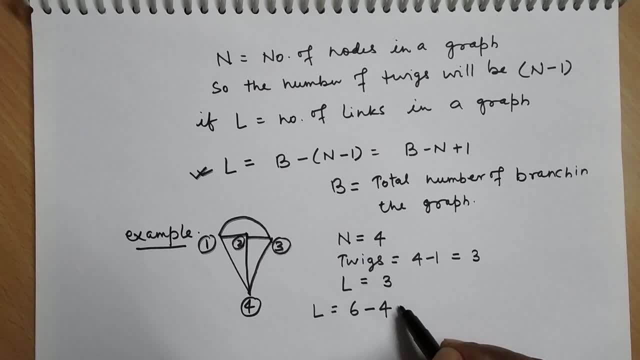 L equal to total number of branch 6. L equal to total number of branch 6 minus number of nodes. that is 4 plus 1 minus number of nodes. that is 4 plus 1 minus number of nodes. that is 4 plus 1. 6 minus 4 plus 1 is 3, so there's 3 is. 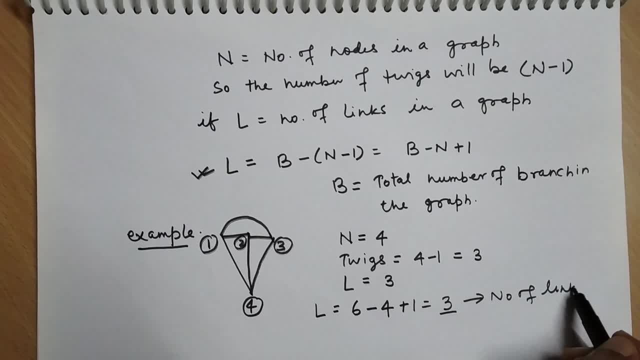 6 minus 4 plus 1 is 3, so there's 3 is 6 minus 4 plus 1 is 3, so there's 3 is number of links now. let's take some number of links now. let's take some number of links now. let's take some examples and draw the nodes and branches. 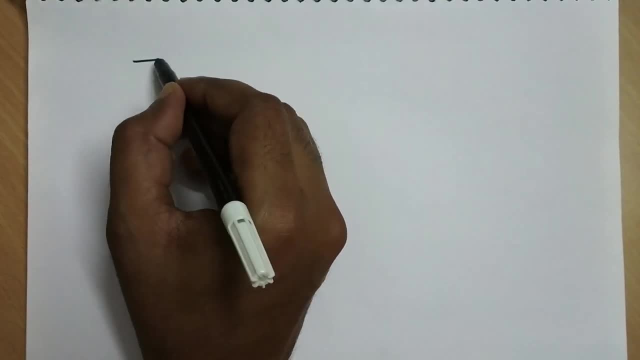 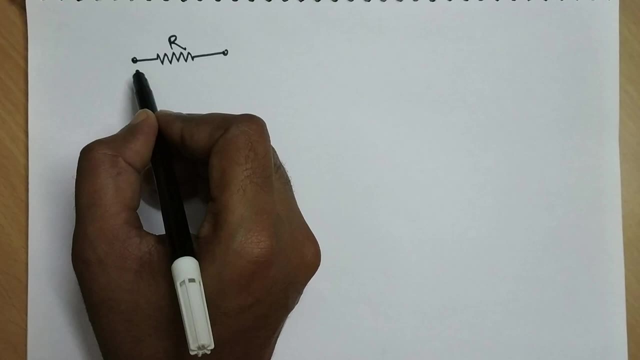 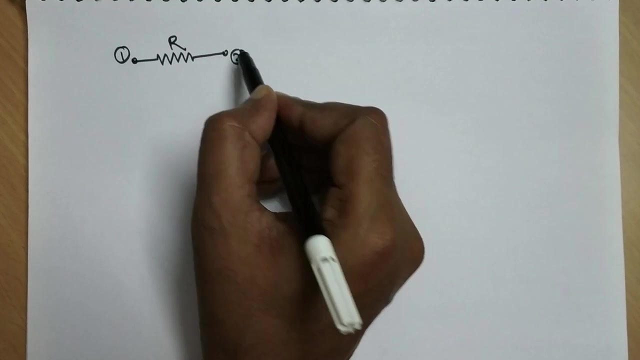 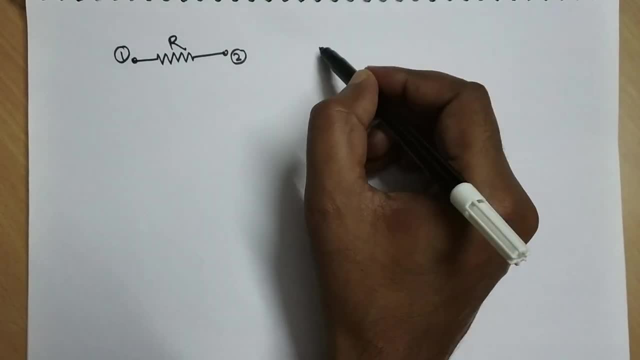 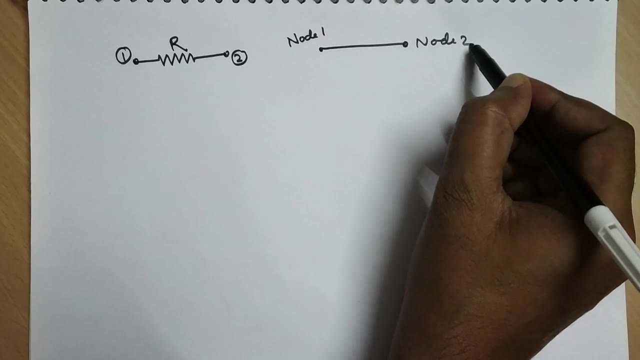 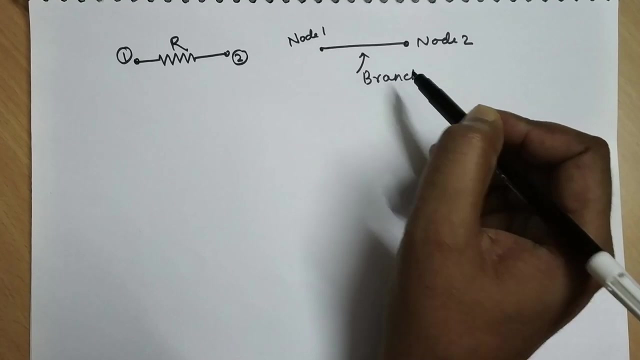 1, not number 1. node number 2. so we can 1, not number 1. node number 2. so we can write this as node 1, node 2 and this write this as node 1, node 2 and this write this as node 1, node 2 and this will be branch. 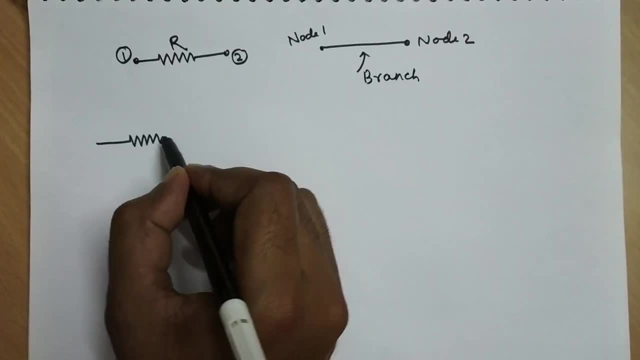 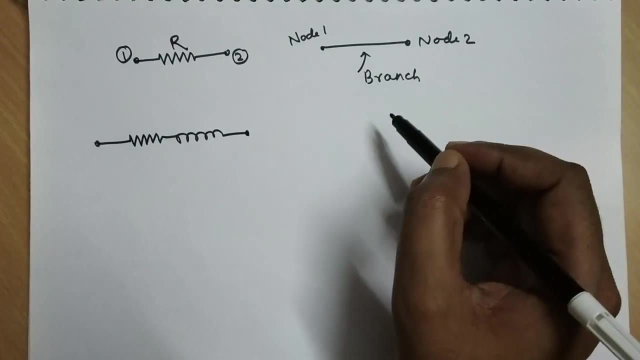 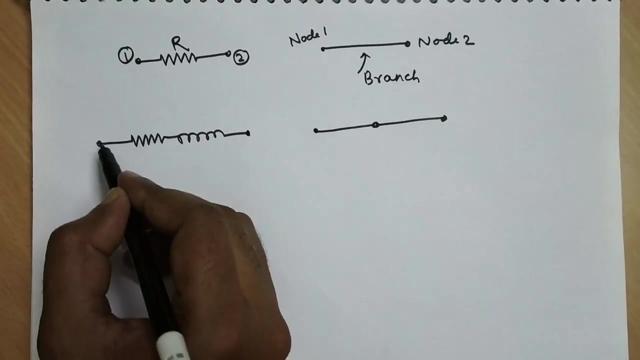 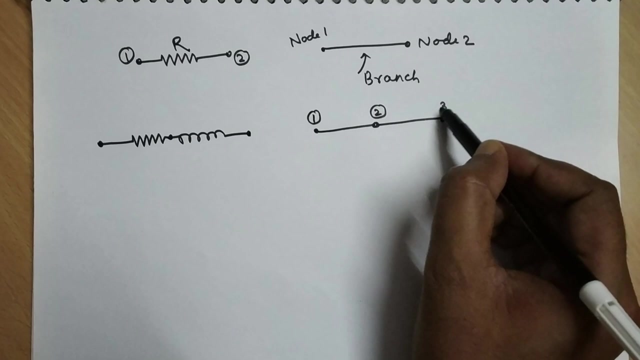 will be, branch will be branch. let us take two elements in series. so there will be three nodes, one, two, and so there will be three nodes, one, two, and so there will be three nodes, one, two and three: node 1, node 2 and node 3. this is 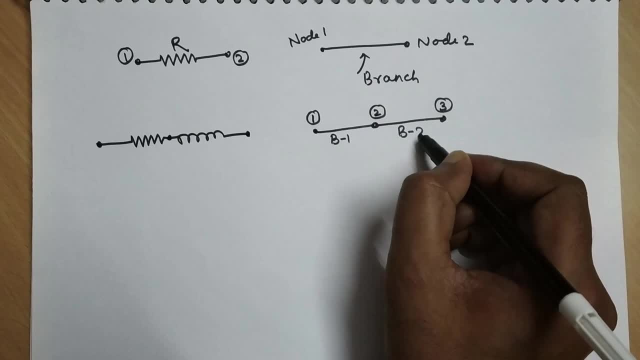 three: node 1, node 2 and node 3. this is three: node 1, node 2 and node 3. this is branch 1. branch 1. branch 1. this is branch 2. let's take a parallel. this is branch 2. let's take a parallel. 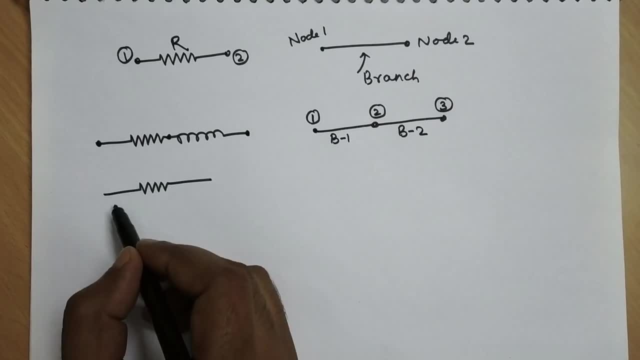 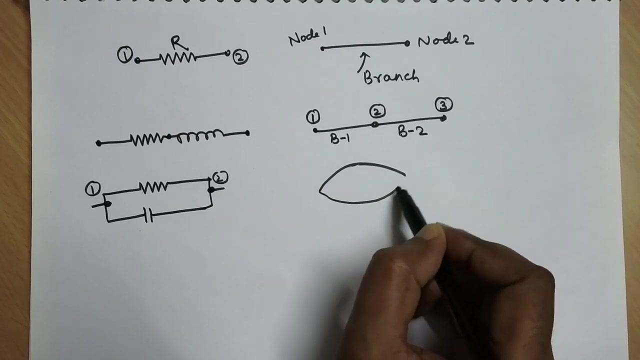 this is branch 2. let's take a parallel combination and there will be only two nodes in the and there will be only two nodes in the and there will be only two nodes in the parallel connection and we can convert parallel connection and we can convert parallel connection and we can convert that in this way: node 1 and node 2, this 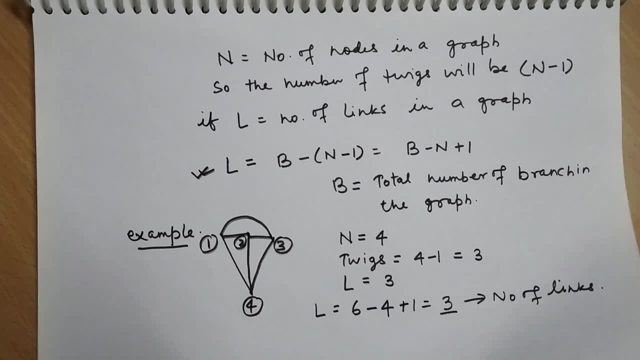 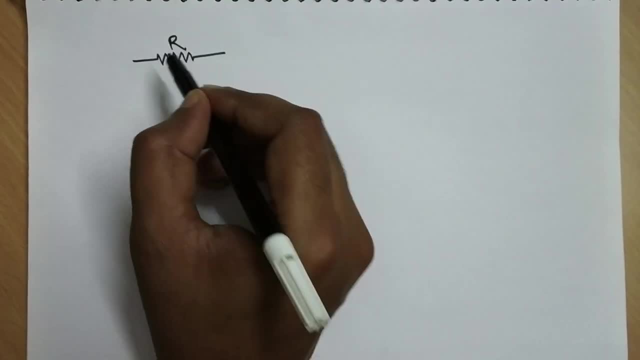 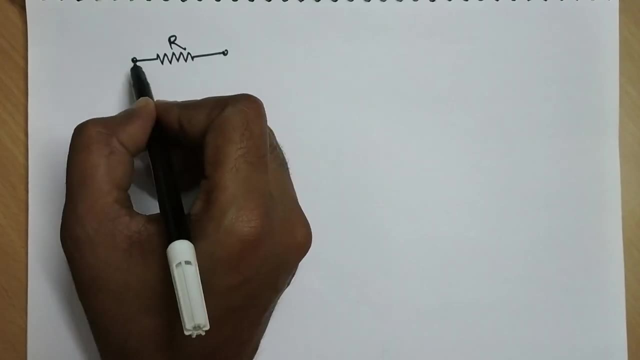 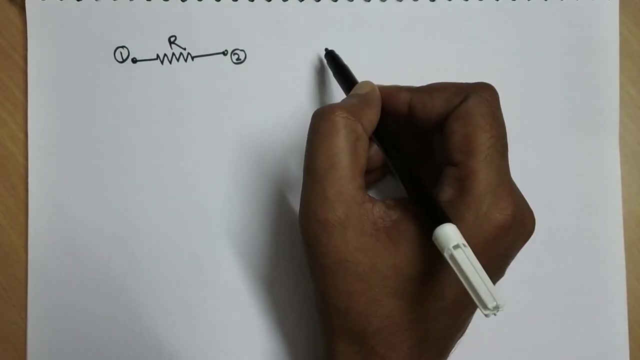 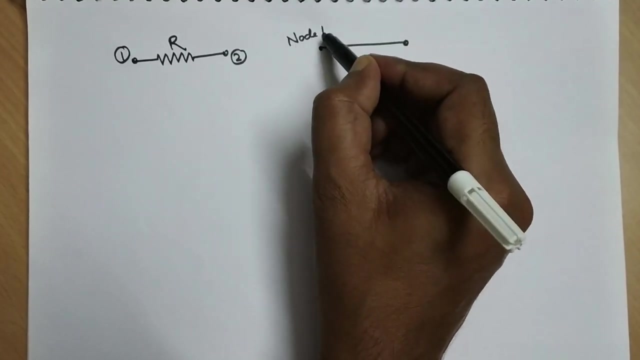 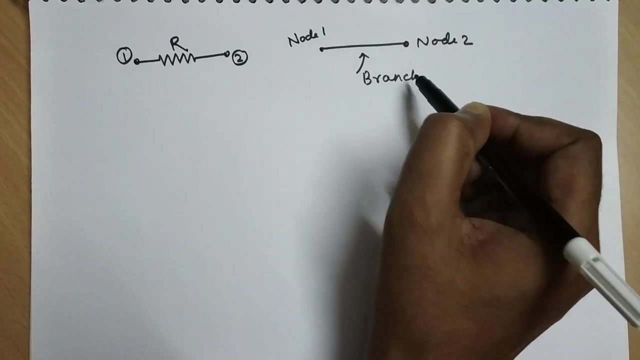 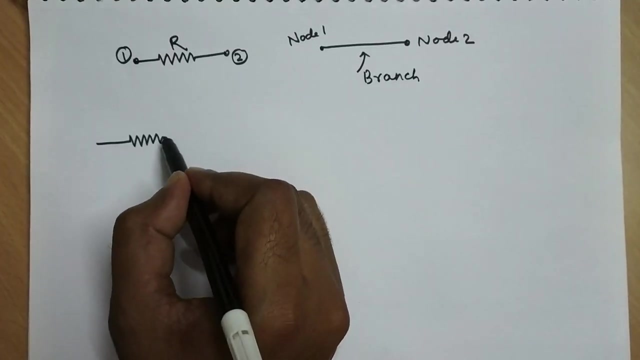 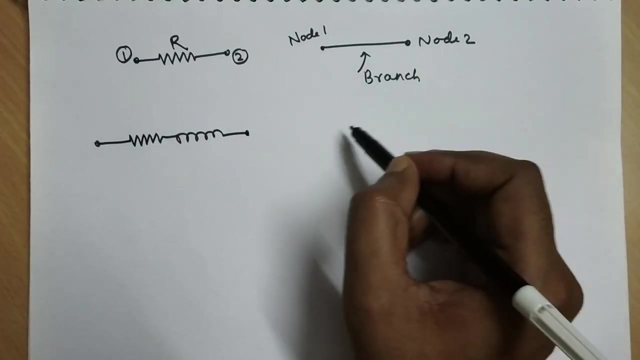 Now l will take some examples and draw the nodes and branches of the network element. So here, total number of nodes in this is 1, node number 1, node number 2.. So we can write this as node 1, node 2, and this will be branch. Let us take two elements in series. 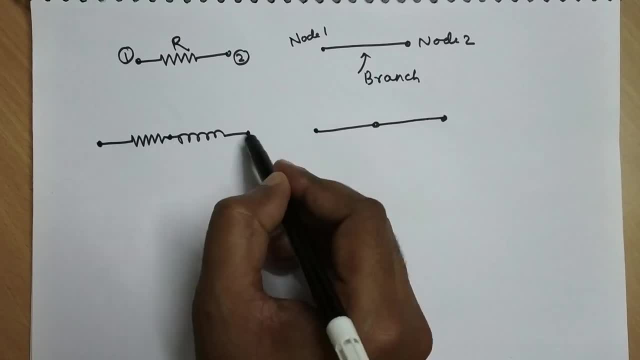 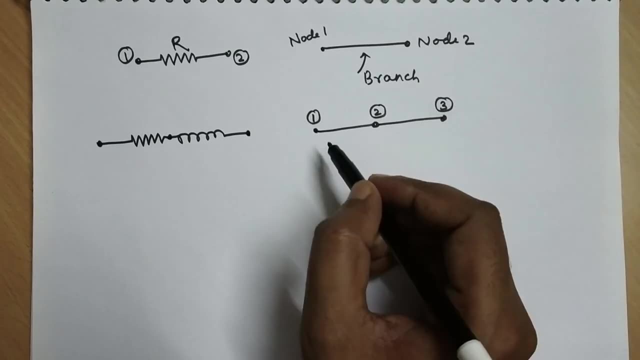 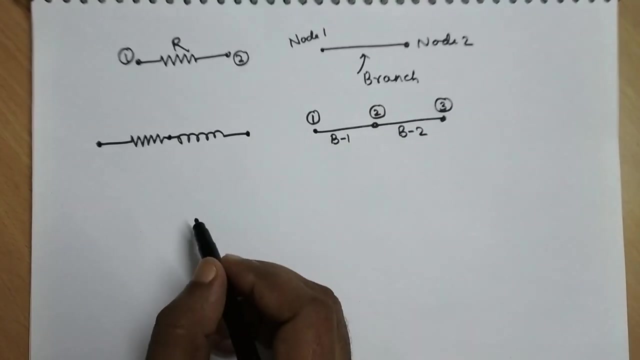 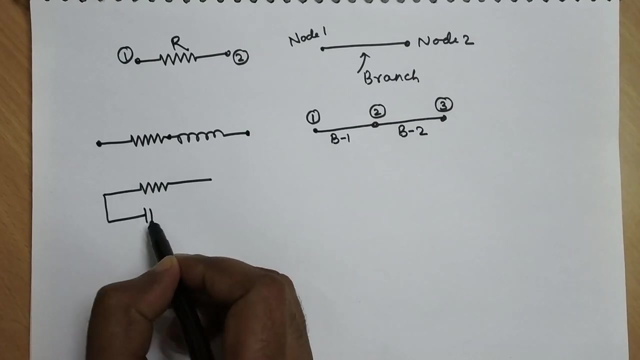 So there will be 3 nodes: node 1, node 2 and node 3.. This is branch 1, this is branch 2.. Let us take a parallel combination and there will be only two nodes in the parallel connection and we can convert. 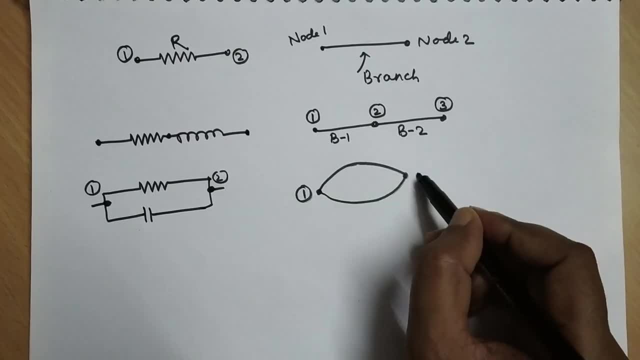 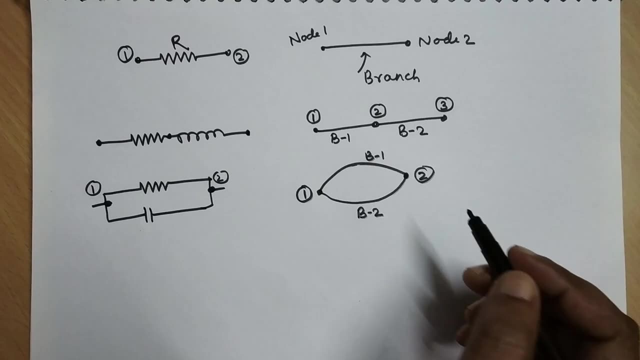 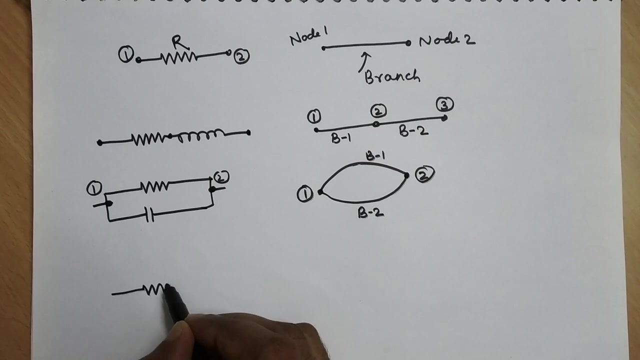 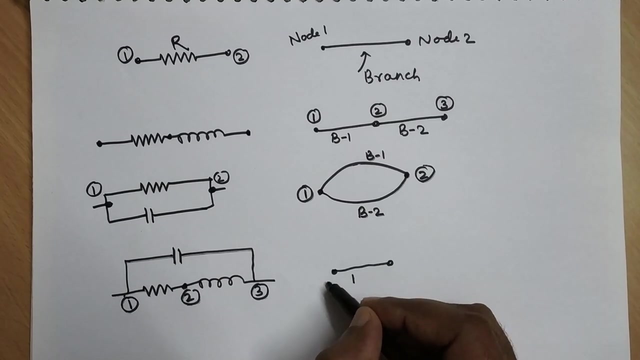 that in this way, node 1 and node 2, this is branch 1 and branch 2. now in this example we have one, two and three, three nodes. so we can make it like this: node 1, this is branch 1, node 2, node 3, branch 2. 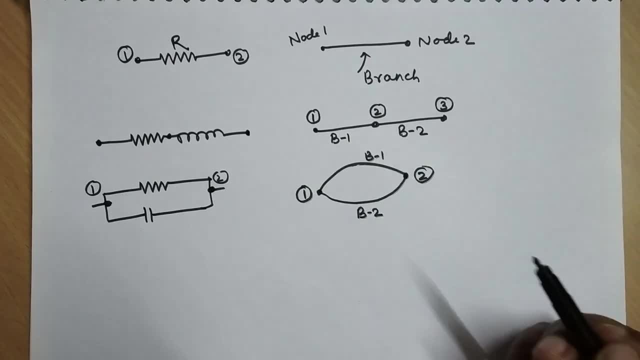 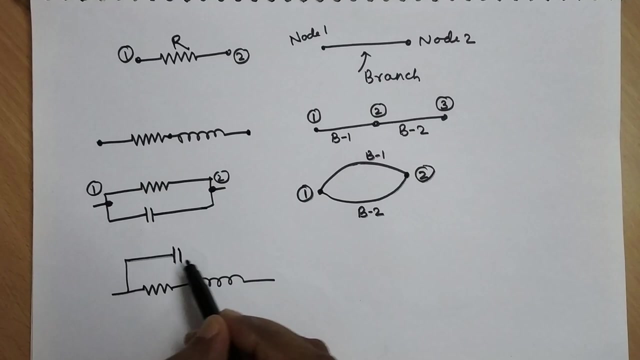 that in this way, node 1 and node 2. this that in this way, node 1 and node 2. this is branch 1, is branch 1 and branch 2. in this example, we have 1, 2 and 3, 3. in this example, we have 1, 2 and 3, 3. 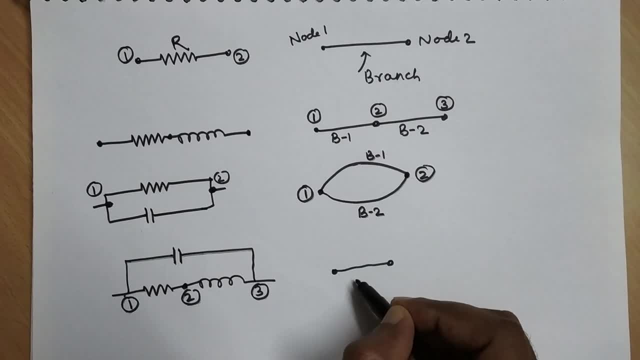 in this example we have 1, 2 and 3, 3 nodes. we can make it like this nodes. we can make it like this nodes. we can make it like this: node 1: this is branch 1, node 2. node 3, branch 2. 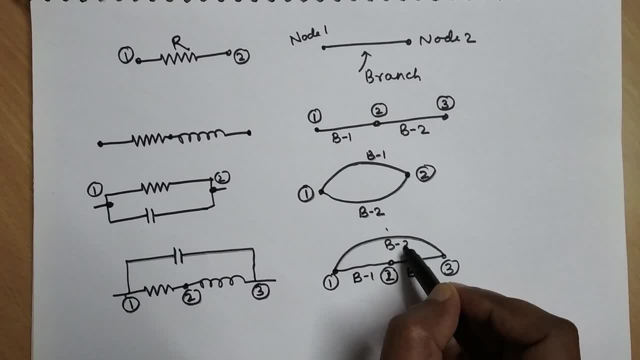 node 1: this is branch 1. node 2, node 3, branch 2: node 1: this is branch 1. node 2, node 3, branch 2, and then branch 3, so this is, and then branch 3, so this is, and then branch 3, so this is how we can convert any network into its. 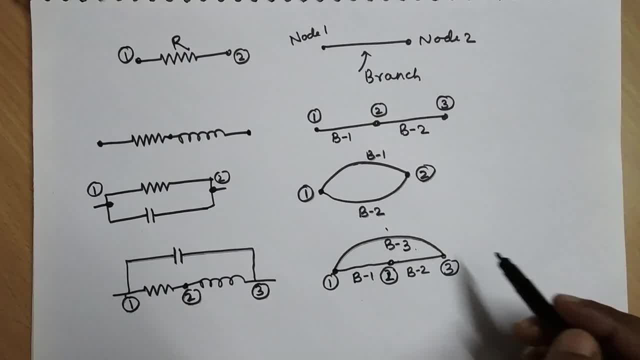 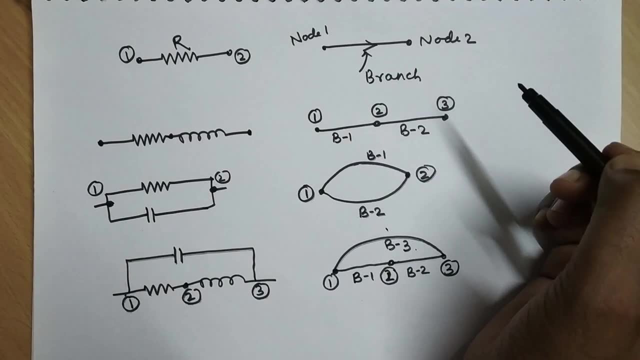 how we can convert any network into its, how we can convert any network into its graphical form. after converting to graphical form. after converting to graphical form. after converting to graphical form, we can assign the graphical form. we can assign the graphical form. we can assign the direction of current. we can assume any. 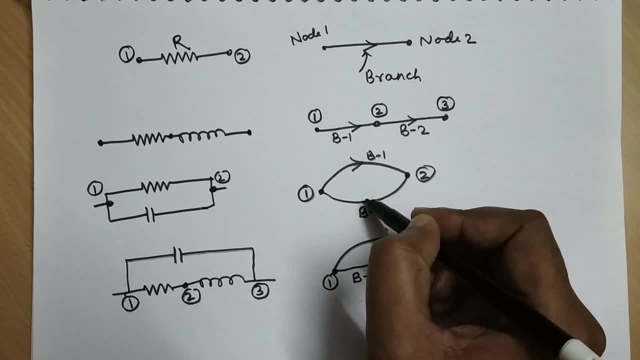 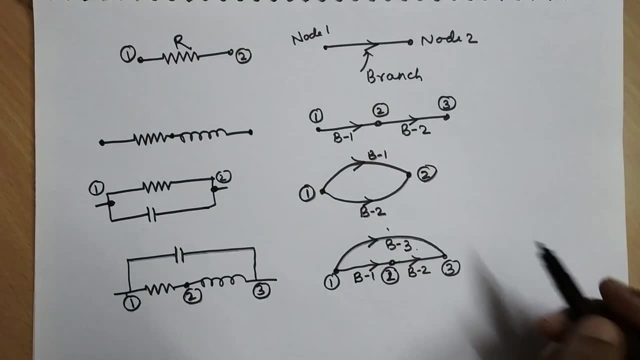 direction of current. we can assume any direction of current. we can assume any direction of current and this type of direction of current and this type of direction of current and this type of graph in which the direction is assigned- graph in which the direction is assigned, graph in which the direction is assigned- is called oriented graph. oriented graph. 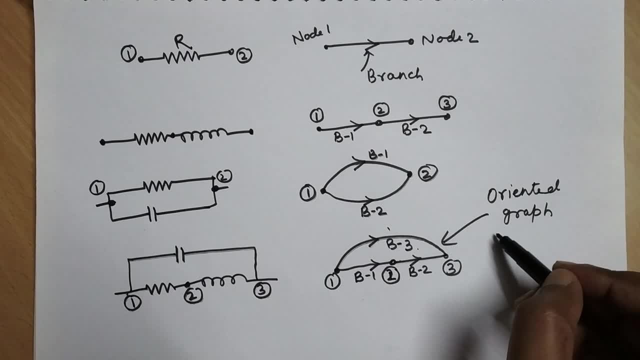 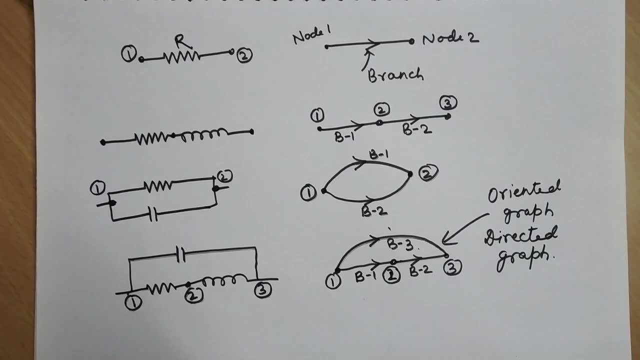 is called oriented graph, oriented graph is called oriented graph, oriented graph, or it's also called directed graph, or it's also called directed graph, or it's also called directed graph. so in these four graphs we can see in all. so in these four graphs we can see in all. 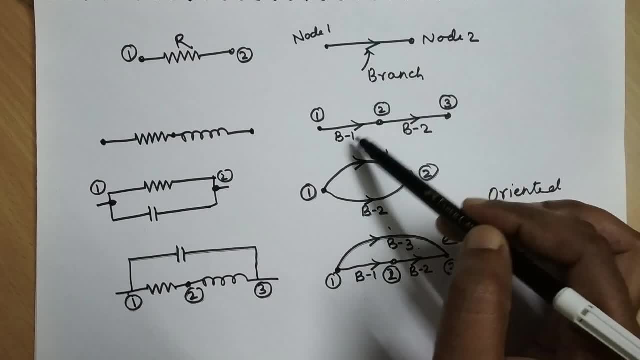 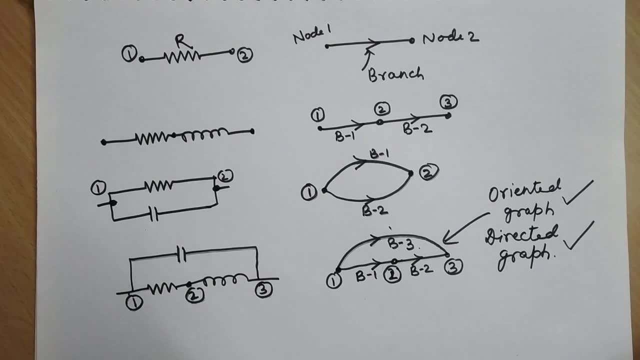 so in these four graphs we can see, in all the elements I have assigned the, the elements I have assigned the, the elements I have assigned the direction of current. so this graph is direction of current. so this graph is direction of current, so this graph is called as oriented graph or directed.